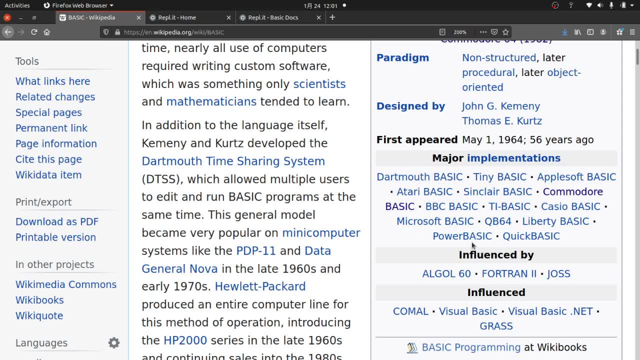 And certain languages had certain features. For example, I think Apple had more graphics features, whereas the Commodore Basic had no graphics features. So it's really, it really really varied, And I started out with what's called Sinclair Basic on what our British friends would call ZX81.. 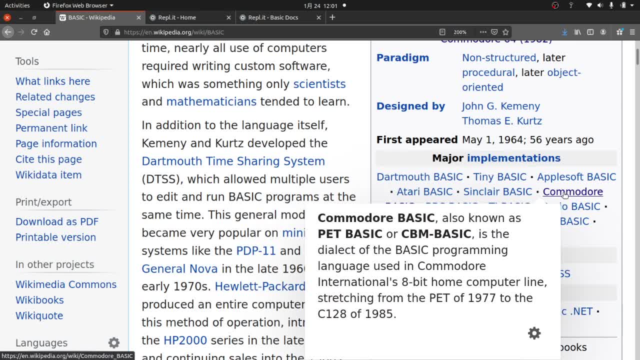 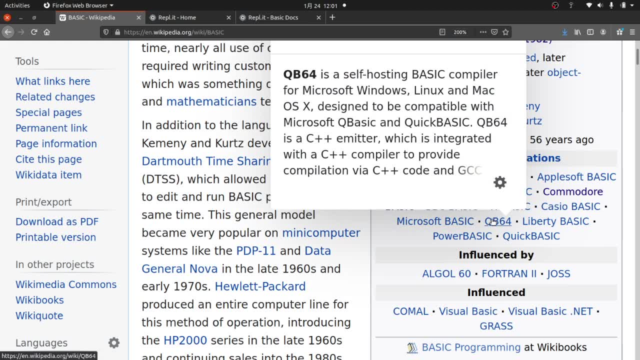 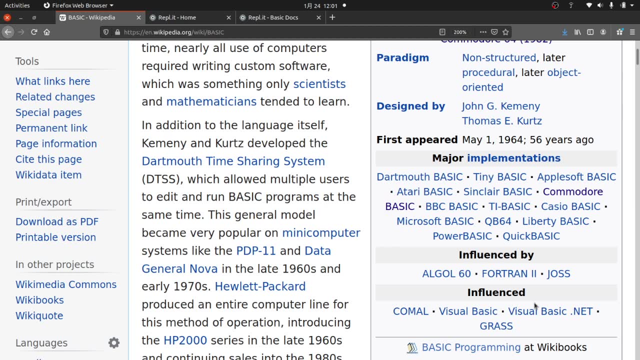 It was a Timex Sinclair 1000 in the United States. Then I had a couple Commodore computers. Then later I learned about QBasic And there is still- There's still- a version of that floating around as well. There's also Visual Basic. that came along later and just really expanded what the language could do. 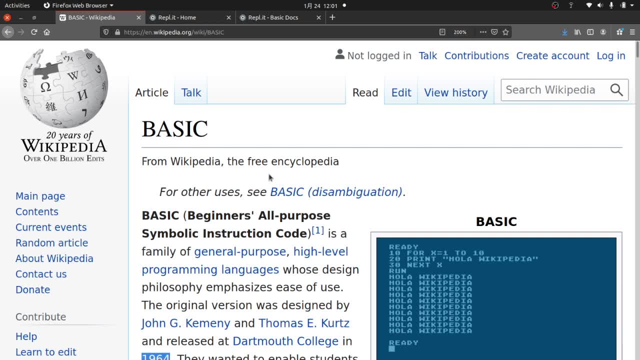 So today, what I want to do is just kind of give you a real quick overview of what classic old school basic was like, And you'll see that it. you know, while it was easy in some ways for beginners, it was also taught a lot of bad habits and had a lot of limitations. 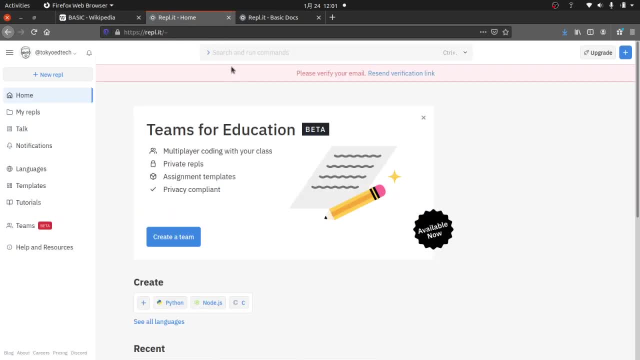 So what I'm going to do is I'm going to click over to here And I'm using website REPLit. so REPLit, And this is a great website. You can create a free account. You do have to sign up, though. 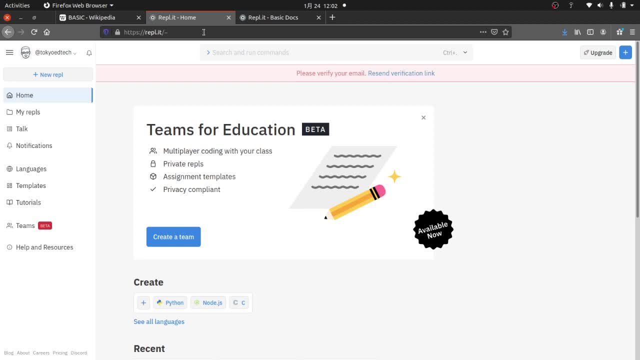 It's, it doesn't? it used to let you just kind of program without an account, but now they require you to sign up And it's definitely worth doing So. once you get into REPLit you should see something up here like New REPL. 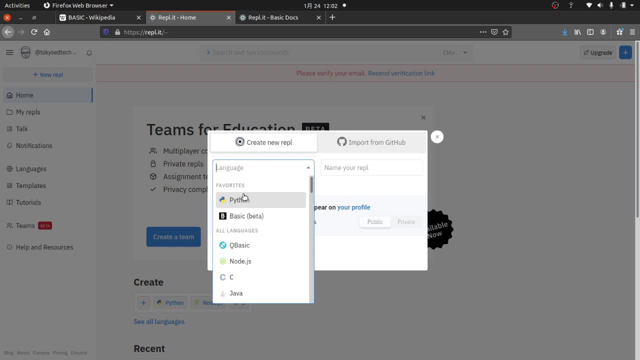 And if they click that, you can choose a language. Now, this does Python, It does well, you can see. it does Basic, It does basically, frankly, every language conceivable. Now, of course, it doesn't do everything in the browser, because that's just wouldn't be possible. 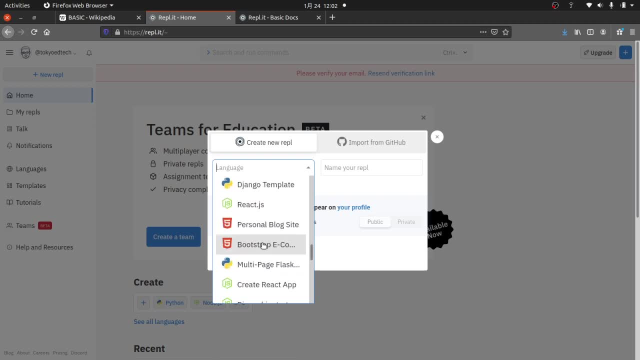 But it does do quite a lot of things. It's really an amazing website and probably well worth the. I think it's four or five bucks a month to join, But you can still use it for free as long as you create an account. 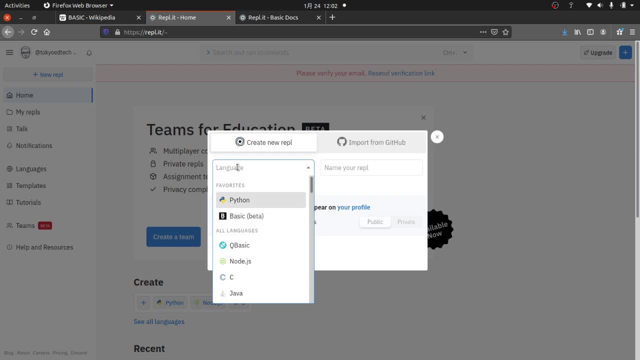 Now you can see I've already been doing Python and Basic. So if you haven't done Basic, just go ahead and type Basic and you'll see three choices: QBasic. QBasic, which is something from the DOS era And again still exists. 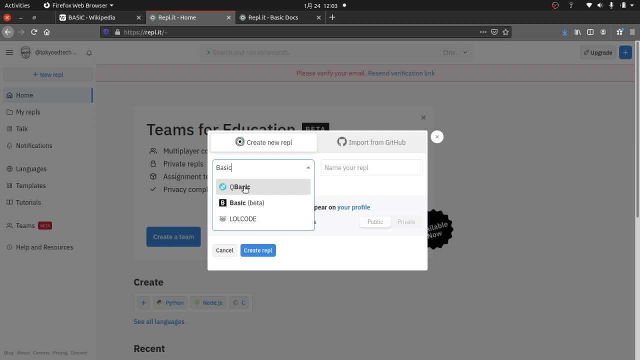 There's still an active user base making- I think it's called QB64 now- And then there is Basic, which is just some people made, and they have integrated it here into REPLit. So let me go ahead and try that out. And this is going to be: you go ahead and create your REPL. 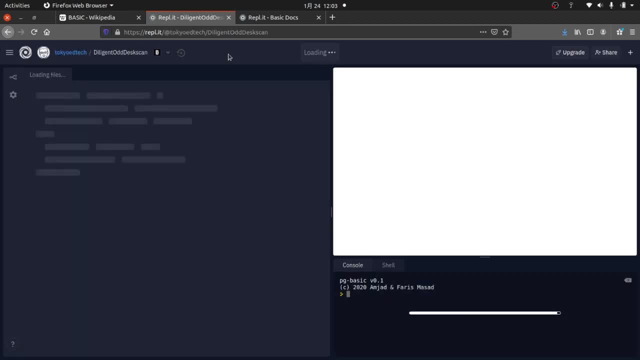 And if you don't have a paid account, it's going to be public. So anybody that has this link Can come in and see what you've been doing. They can't- I don't think they can- change it, but I think they can see it. 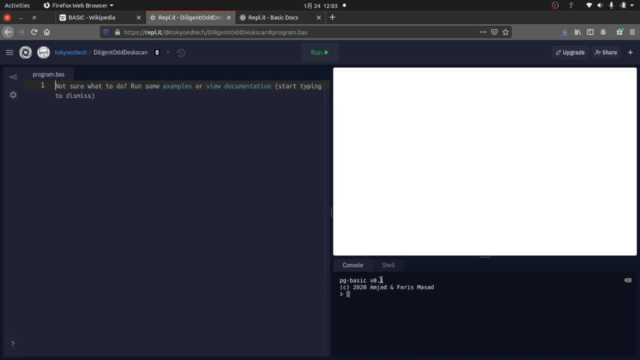 So this is called PG Basic and this is version 0.1 by Amjad and Faris Masad. So thank you very much to those people for creating this and sharing it with the world, And I'll see if I can get a link to that down below as well. 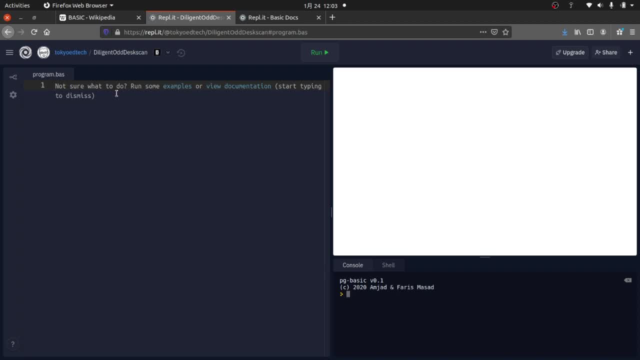 So let me talk to you about Basic And again, this is old school Basic. There are newer, updated versions that are more modern, Have more modern features, But this is the old school Basic that people used. You know. they said, like I said, my generation- late 70s, early 80s, the 8-bit golden era. 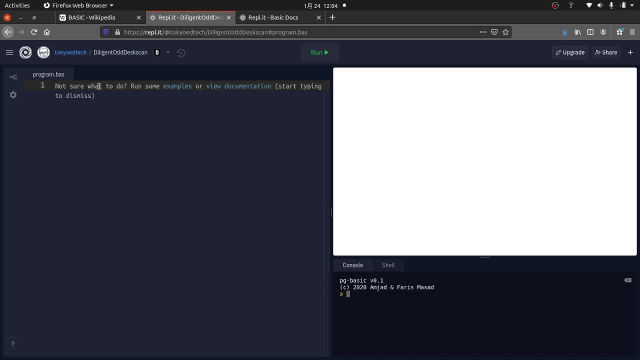 So Basic started out with something called line numbers. So you had to actually number every line of your program And the general convention was to do your line numbers every 10.. And I'll show you why in a second. So the first thing I'm going to show you is how to do a comment. 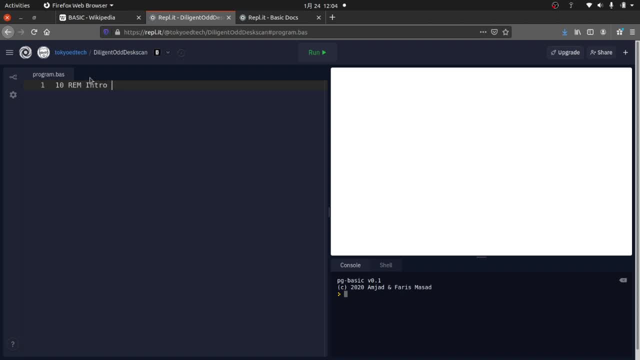 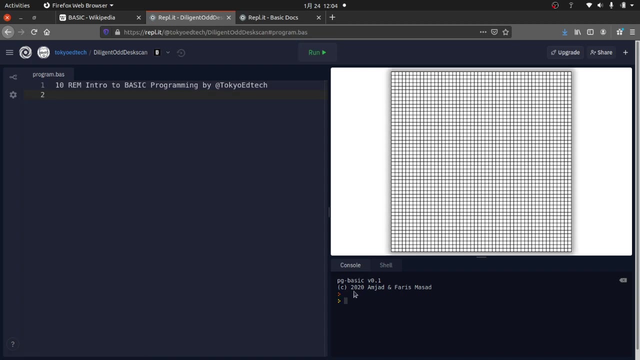 So I don't know. I'm going to say, you know, intro to basic programming by Tokyo Ed Tech, And that is me. Now, if I run this, you'll see nothing happens. So this is a comment. So if this was a Python program, it would be a hashtag. 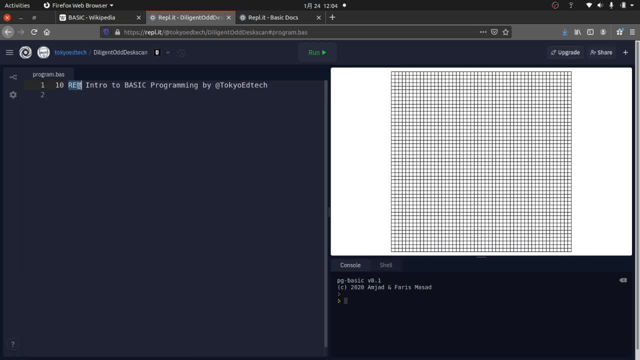 But it is a basic program And we use REM, And this is just a note for the programmer, So it doesn't actually do anything. So the first command I'm going to do is print. So print, And then you don't need parentheses or anything. 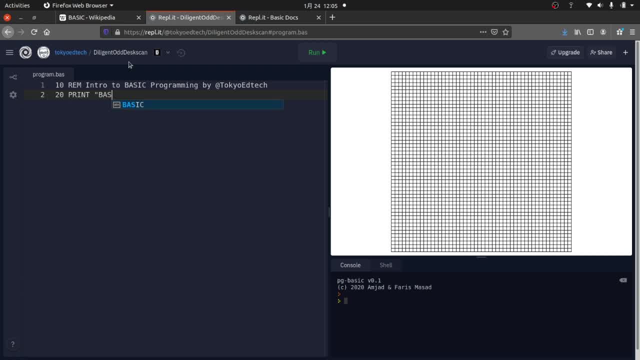 Just type: I'm going to put Basic- say Basic Programming for Beginners- by at Tokyo Ed Tech. Now you'll notice I'm capitalizing all of the basic keywords. This was just kind of the way it was done. Now this particular interpreter doesn't care. 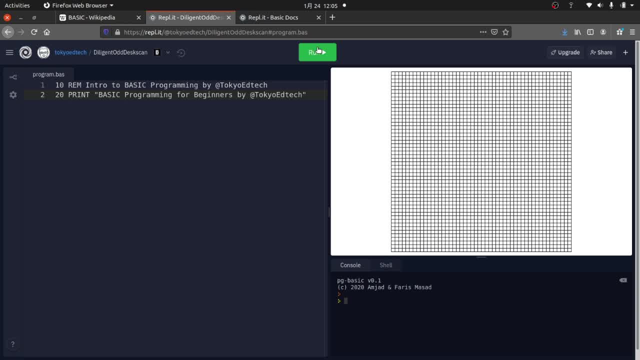 You can do lowercase, You can do uppercase, It doesn't matter, But I'm going to do it uppercase just to keep it kind of old school. So now, if I run this And you can see now Basic Programming for Beginners by at Tokyo Ed Tech. 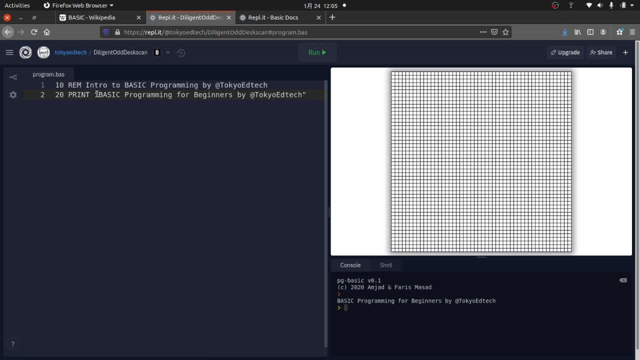 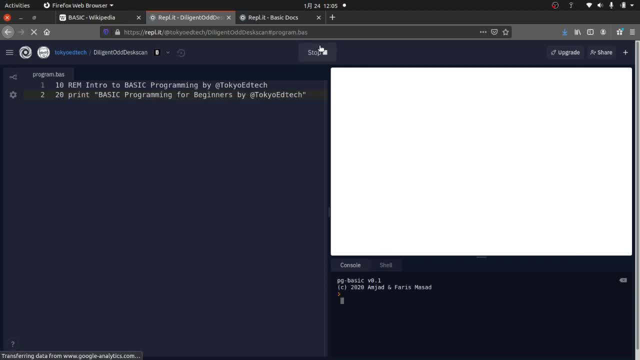 So this is our print statement And this is very similar, of course, to how Python does it And you just do print Again this interpreter. I can do lowercase if I want, But I'm kind of having a little walk down memory lane here. 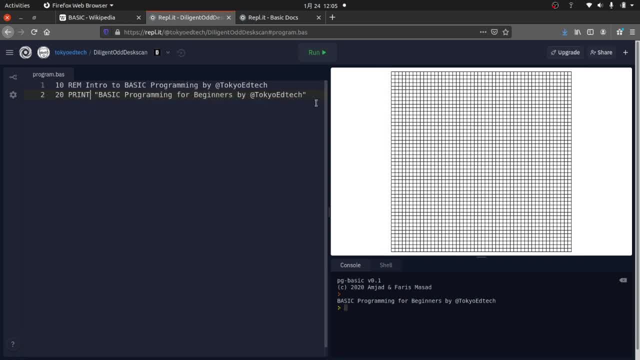 So I'm going to do it in capitals, And yeah. So that's the statements. Now notice I'm skipping every 10.. I don't have to do that, But I am doing that because, the reason being that, if I go back and I go, oh my gosh, I forgot to put something. 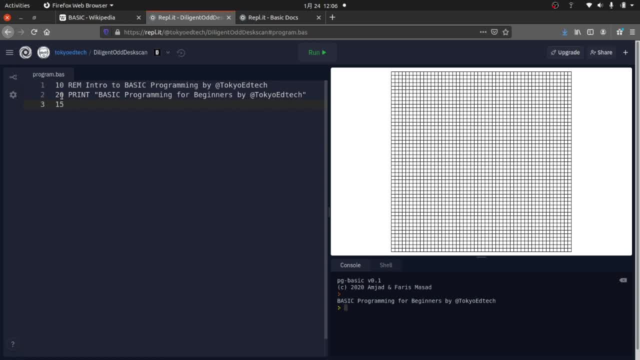 Then I can go ahead and put line 15 in the middle And then I can add something above and below that. That was kind of the logic behind that. Now there is in most versions of Basic. there is a command called. So let's say, I wanted to. 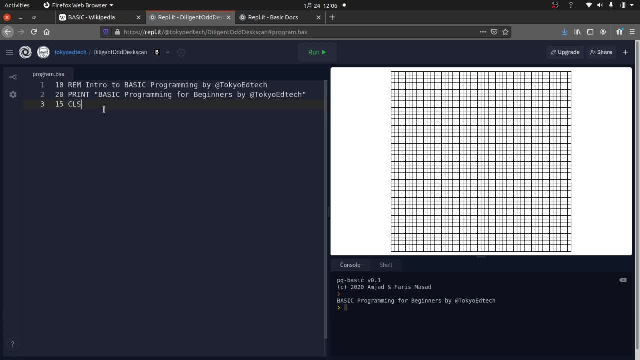 Clear the screen, And that was going to be line 15.. But I'm going to leave that out. It doesn't actually work in this one, At least I don't think it does, Or I haven't noticed that it does. But let's just leave that out for now. 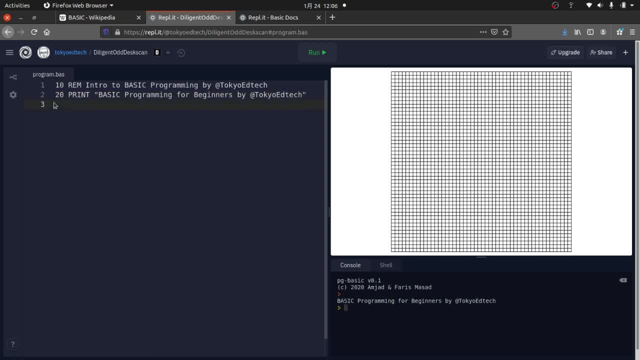 We don't really need that, But there is a clear screen command. So let's move on and do integers, Integers and floats, And so, again, if you're a Python person, you know what a float is. So In Basic we do let 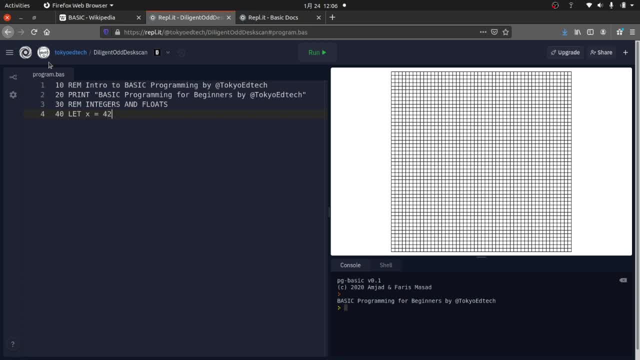 So, for example, let x equal 42. Now, in this case, x would be an integer. Now, this is one of those areas where the programming language, This programming language or version of Basic, differs from, say, Commodore Basic. So if this was Commodore Basic, I think you had to do. 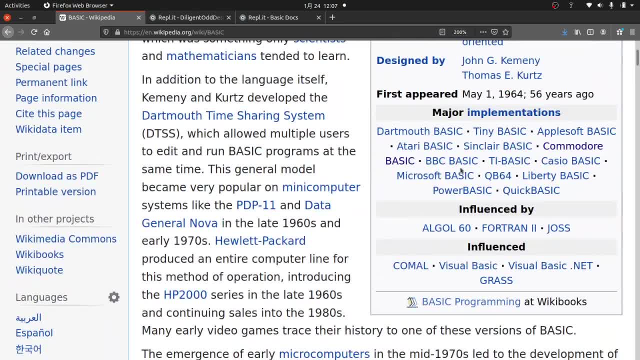 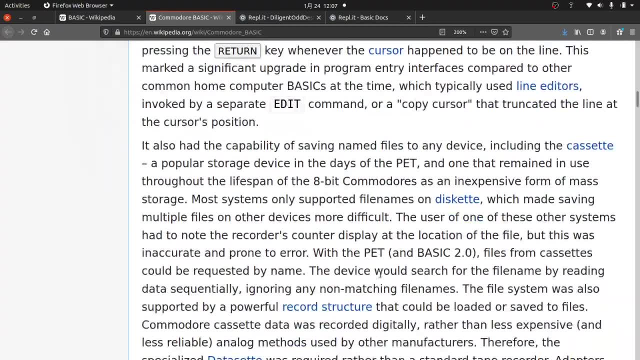 What was it? I just actually looked at it and of course forgot In Commodore Basic you had to do something with To let it know it was an integer or a float. Where is it at here, Basic? Yeah, the dollars. 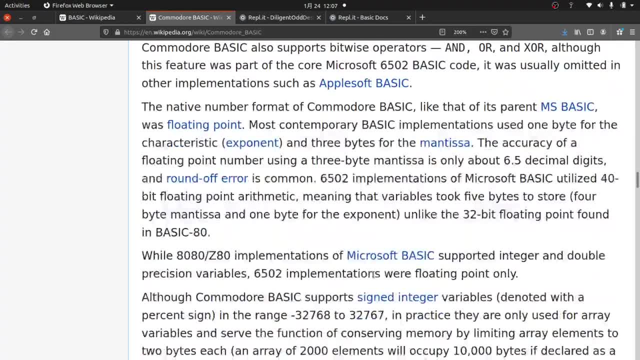 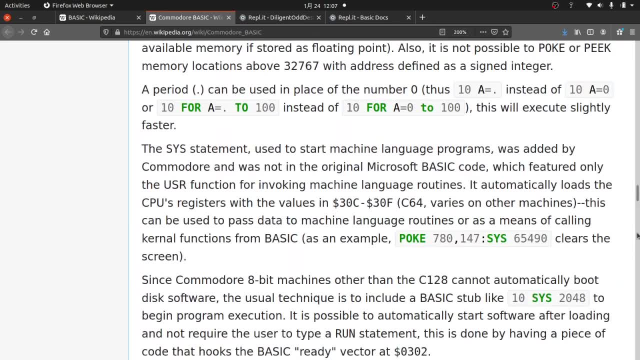 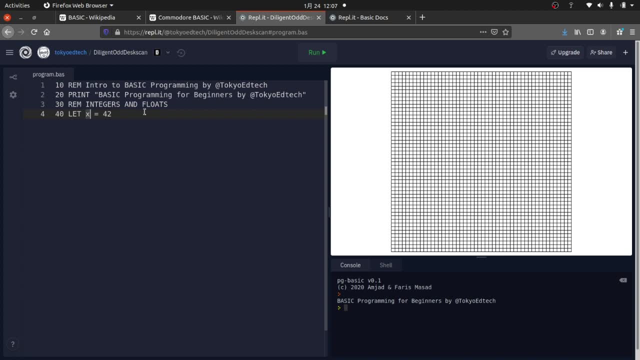 I remember that part And Okay, That's it. Okay, got it. So I didn't know what I was doing. Okey dokey. So in Commodore Basic, which is what I used, If you don't put anything with the variable, it's going to assume it's an integer. 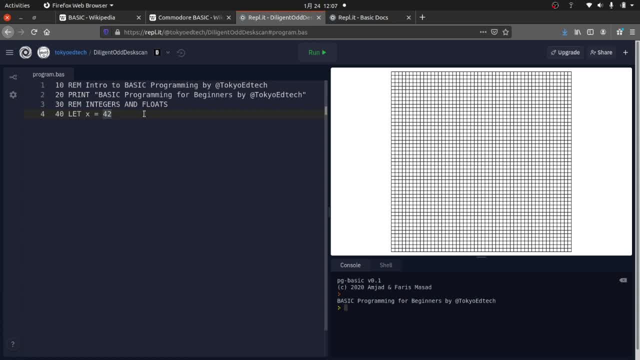 Now in this particular version of Basic it doesn't matter, But it does matter in other versions. So then I can go ahead and type: you know 50,. you know print x. Or I could say 60, print quote. the answer is quote plus x. 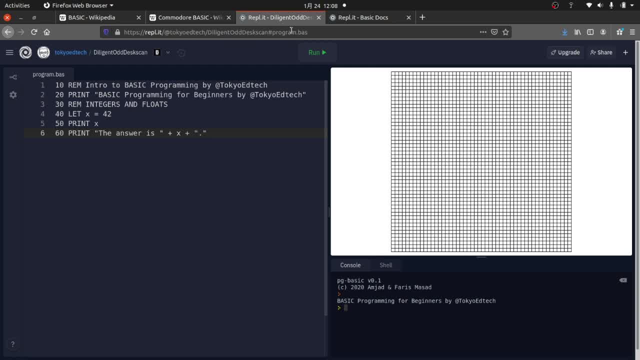 And I could add maybe a little period at the end there. So let's go ahead and run that. Let's see what we get. Okay, So we can print it out just by itself, Or we can print it out as I did here. 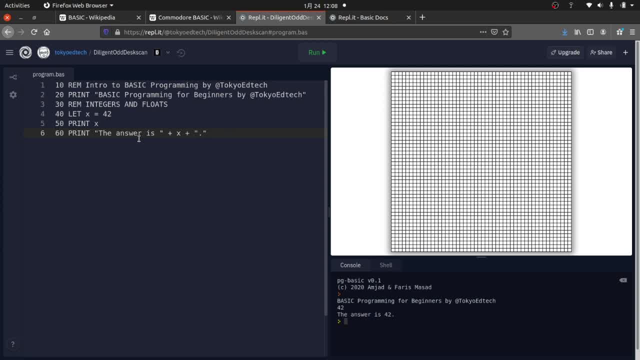 And this is kind of like Java, the way Java does it. And notice, I didn't have to convert this to a string, It automatically converts it for us. So we have a space here. So so far, so good. It's probably very similar to what you've done before. 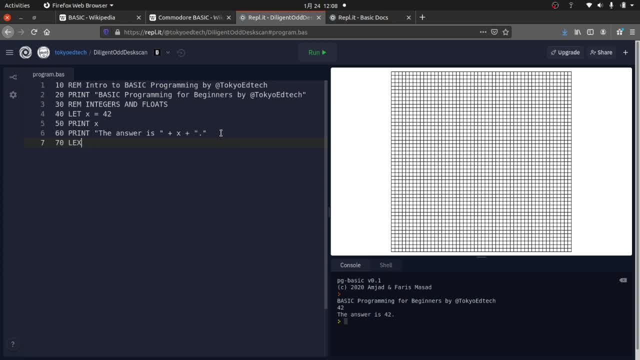 And then I'm going to go ahead and do a float. I'm going to say: let a y equal, Let's say one, Let's say 1.21.. And then now we can see that this is a float. Okay, Again, in Commodore BASIC I have to add a percent. 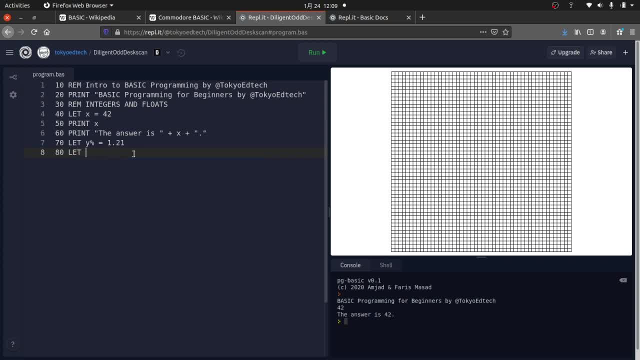 And I wonder if that's going to work. Let's try that. So let's, sorry, print quote: I should say y percent plus gigawatts And see if that works. Okay, So we cannot do the percent with this particular version. 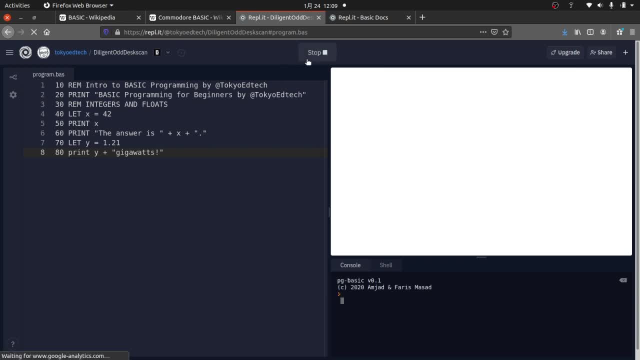 Okay, And of course it doesn't know what percent is there. So go ahead and run And you can see we got 1.21 gigawatts. I'll put a space in there so it looks a little bit better. 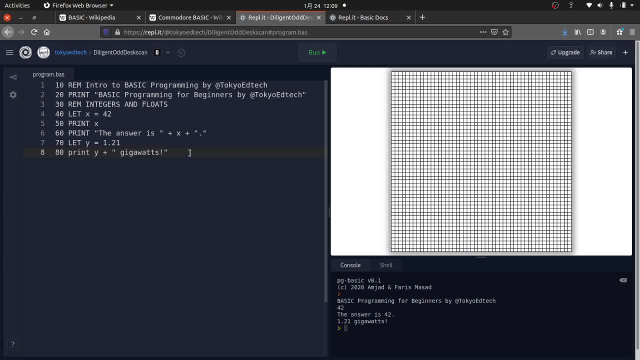 Alrighty, So far, so good. Again, in different versions of BASIC you have to name your variables slightly, But in this version of BASIC it's a little bit more forgiving. So thank you to the developers who were kind enough to make it easy for us. 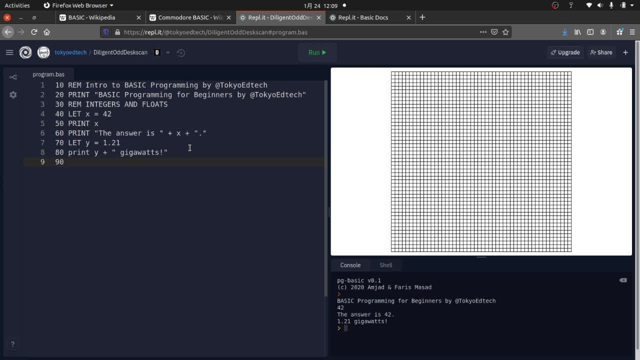 Now there are a number of math functions built into this programming language, So I'm just going to go ahead and do a few for you. So abs, And we could do absolute value of y, We could do print. What else can we do? 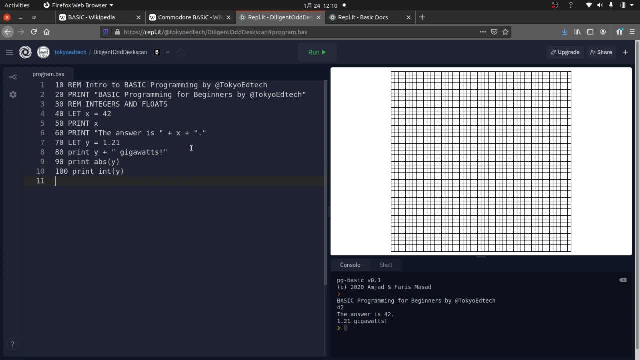 Int y, And in a lot of the older versions of BASIC you would actually use floor instead of int, And what this does is it chops off the decimal point. So I go to run And you'll see 1.21 gigawatts. 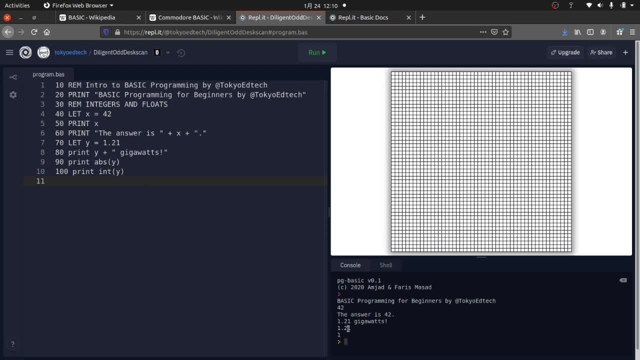 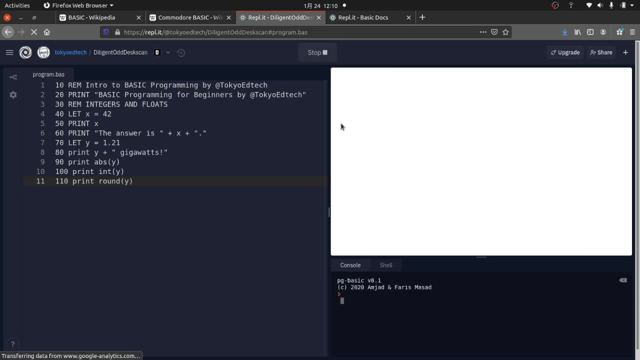 The absolute value of 1.21 is still 1.21 because it's positive, And you can see here how int chops that off to a 1.. However, if we wanted to round it, we could do round y, And now, of course, that's still going to be 1 because 1.21. 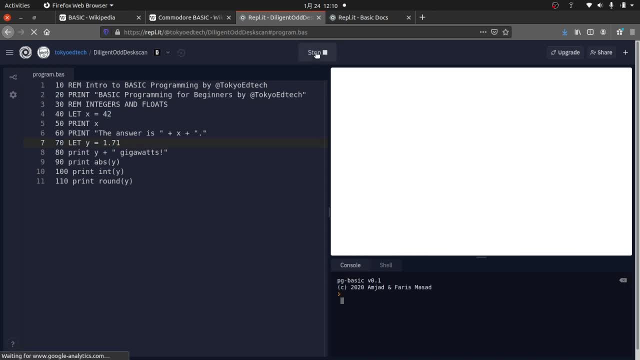 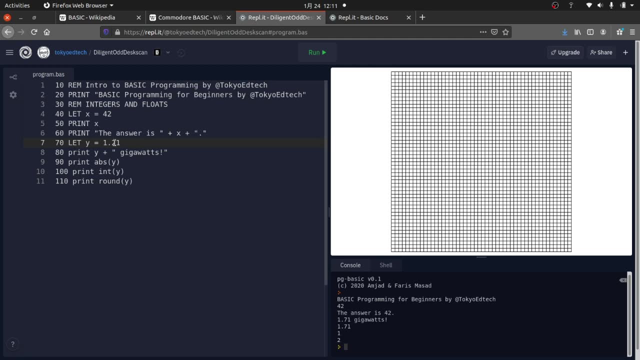 But let's say, if we change this to 7, we'll get a different result. So you can see how that rounded up to 2.. But I'll put that back to 1.21 gigawatts, A very important number in cinematic history. 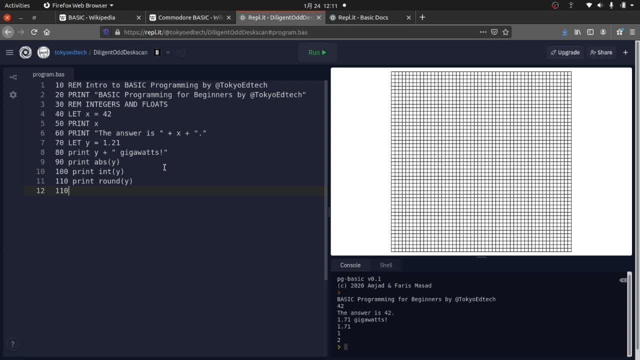 So let's see We also have square root, So 110 print sqr of y. We have random, So I'm going to go ahead and print random. This isn't necessarily about the variables, But it's something you'll use with these things. 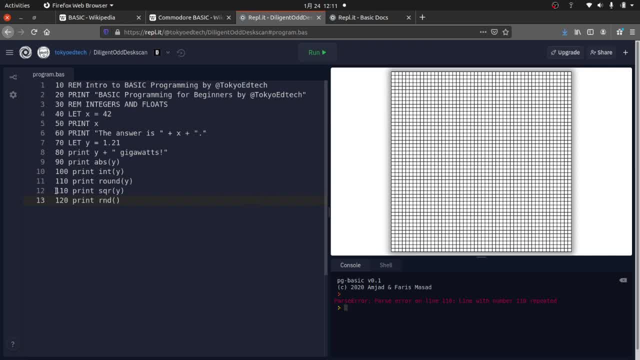 So I'm going to go ahead and run it. Line number 110 repeated. So you cannot repeat a line number. So go ahead and run And you'll see over here that we've got 1.21.. That we've got 1.1.. 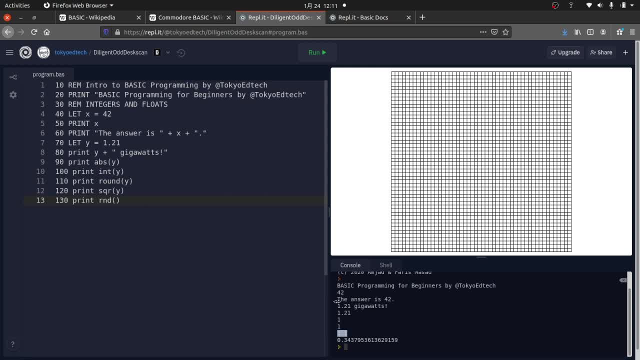 Apparently, the square root of 1.21 is 1.1.. At least very close to that, And then we get a random number. So this rnd is a random number between 0 and 1.. And which we can use later, you'll see. 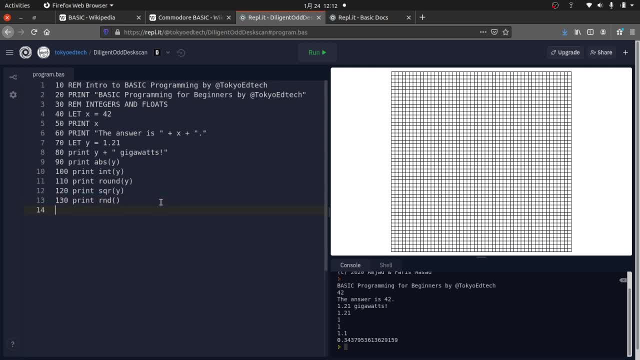 To get a random number, a random integer, And so one more thing we can do Is we can do print val, And what that does Is it converts a string- 3.14 and 1.59.. Into a float. 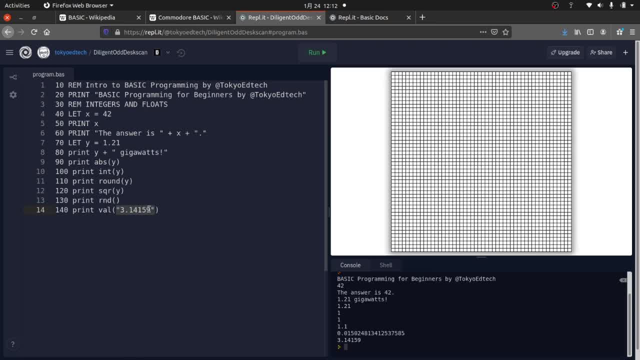 So then what I could do Is then I could multiply that. So this is a case where you're inputting something And you need to convert it to a number. You would use that And then, finally, for this section, We would want to do something along the lines of: 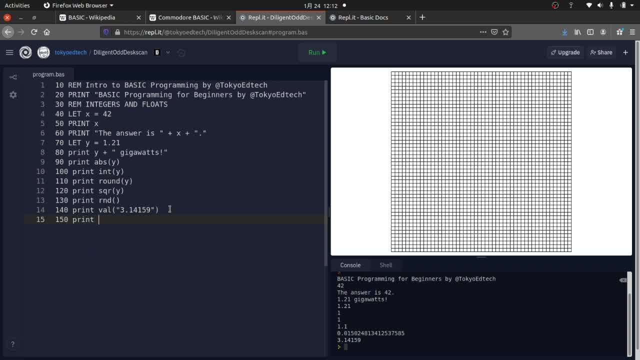 If we wanted a random number, say from 1 to 10.. We would say: print Int, rnd. Remember that's from 0 to .99999.. And we're going to multiply that by 10. And then add 1.. 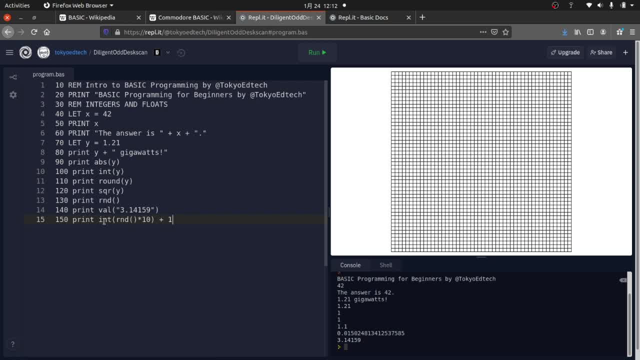 Because what happens is the int cuts off the, You know, cuts off the decimal part, And so it would normally give 0 to 9.. But we want 1 to 10. So we add 1.. So I'm going to go ahead and run that. 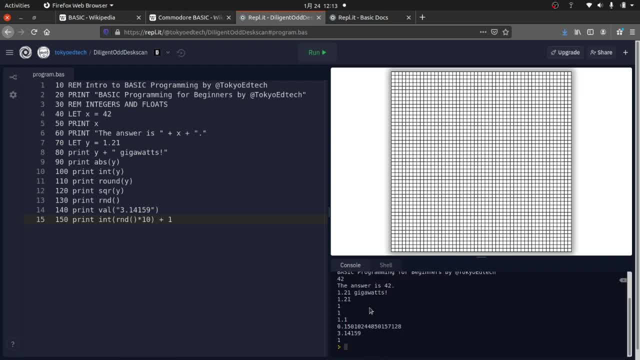 And you see, we got 9.. I'm going to try it again Now. we got 1.. Okay, So you can see we get random values every time. Okay, So moving on, Let's go ahead and do strings, Okay. 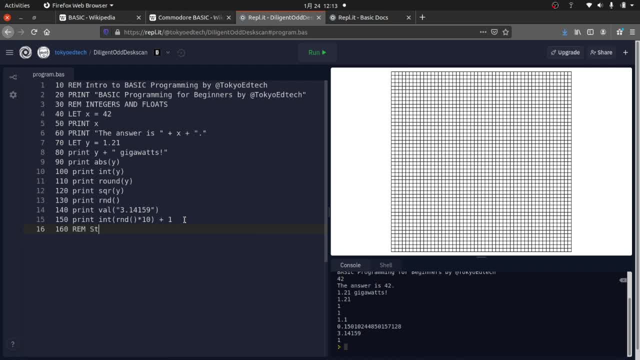 So I'm going to go ahead and do 160.. I'm going to say rem strings, So 170.. So I'm going to go ahead and create a string Now. again I'm going to use let Now in this particular version of basic. 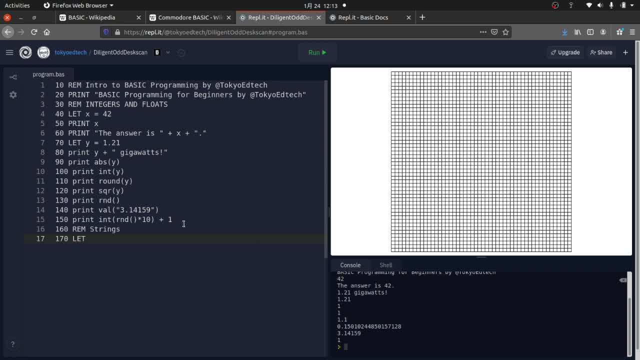 Let is optional, But in a lot of them it is not. So I'm going to say name equals And I'm going to say Tokyo EdTech, because that's me Now again. In Commodore basic you would have to add a dollar sign at the end of that to tell the 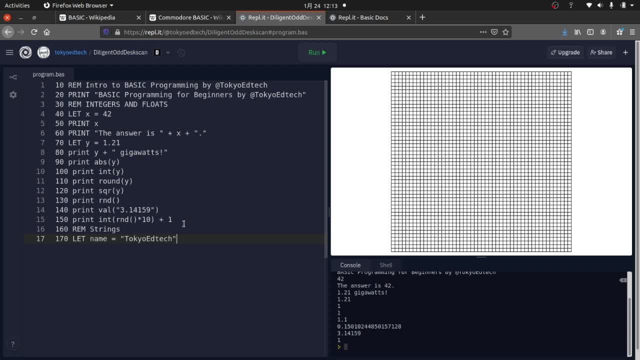 computer. it's a string And that may apply to other versions of basic. Actually, Commodore basic was actually made by Microsoft. A little interesting little story there, How I think it was. Jack Tramiel got a great deal on that. It's very interesting. 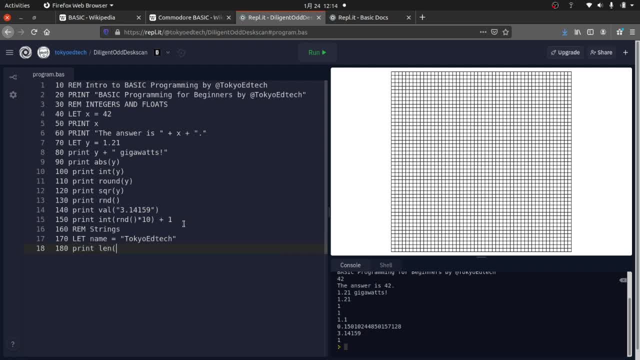 You should look it up sometime So I can do things like print the length of names. So that hasn't really changed since the old days And you can see the length of that is 11.. So 1,, 2,, 3,, 4,, 5,, 6,, 7,, 8,, 9,, 10,, 11.. 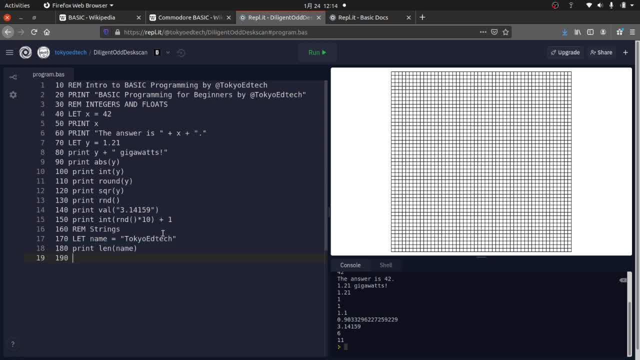 There we go. That's good, That's what we wanted, 190.. We can go ahead and just print. You know, Hi. I'm sorry. You know Hi, My name is Notice. I'm adding plus and then name. 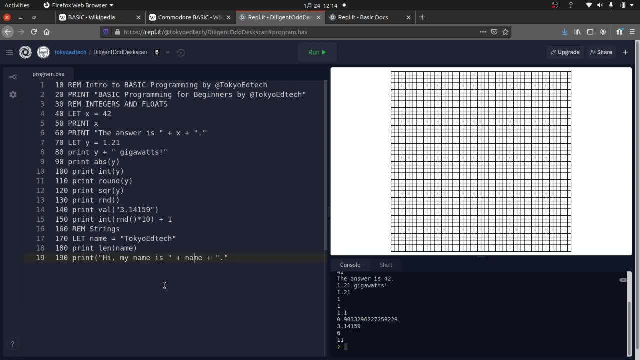 And plus Put the period at the end. I don't need the Parentheses, That's just a habit from doing mostly Python. Let's go take a look And there we go, So we can print that out. So so far it's very. 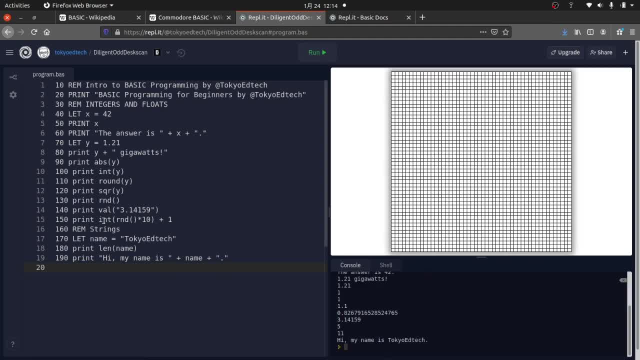 It's especially for coming from, say, Python or something like that. It's probably very, very similar. Now you notice how, just as a habit, I did not capitalize print here, But go ahead and Kick it old school and make it capitalized Again on an older computer. 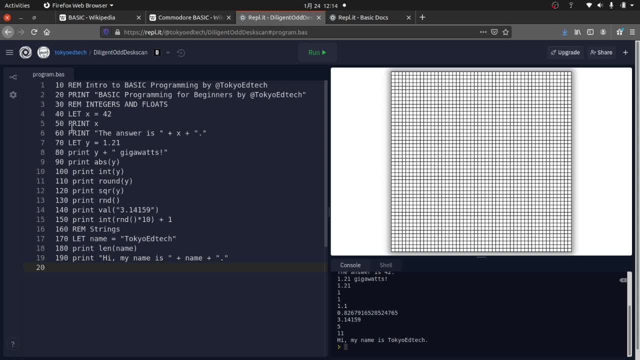 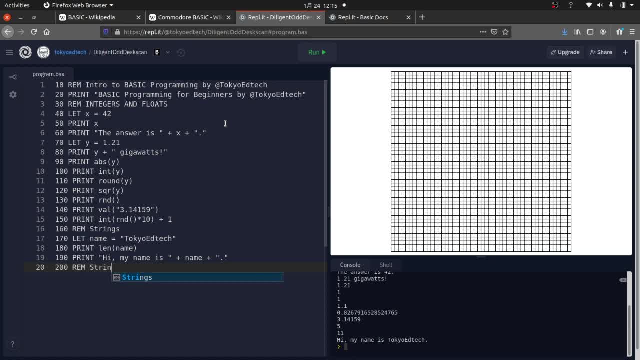 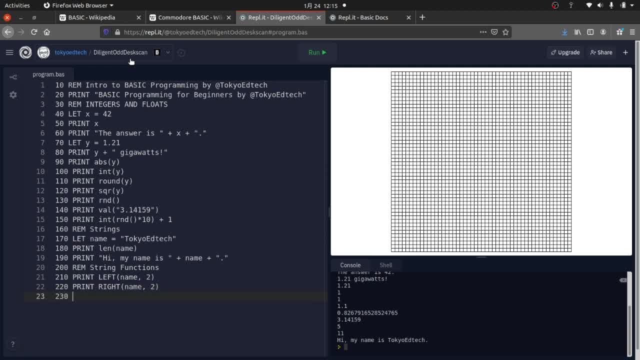 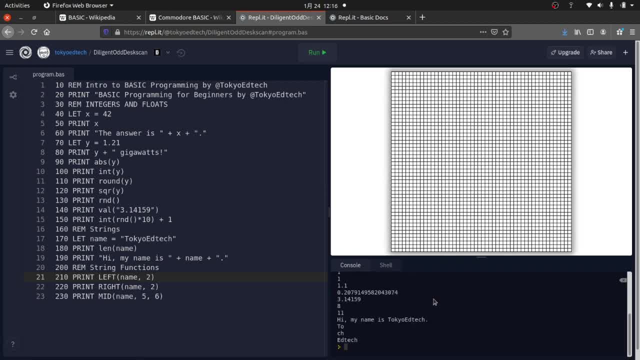 Of Of. Okay, so you can see, here we've got to because it's left. So the left two characters is to the right, two characters is ch, and then we got edtech, So we started at five. So we went from zero. is t, one, two, three, four, five is e, and then six characters. 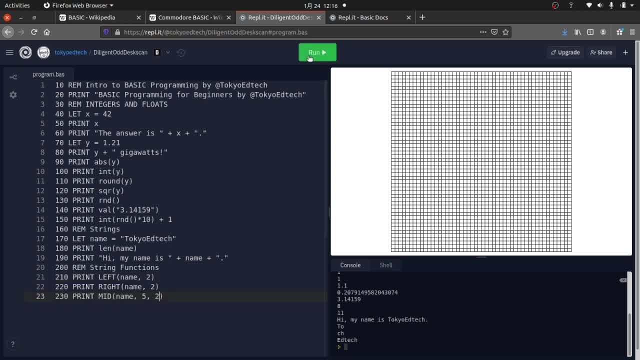 So if I just wanted ed, I would make it like this and you can see: we got ed. So now we could use mid as like substring. or if we want to just pull out a single character, we could do like mid five one. 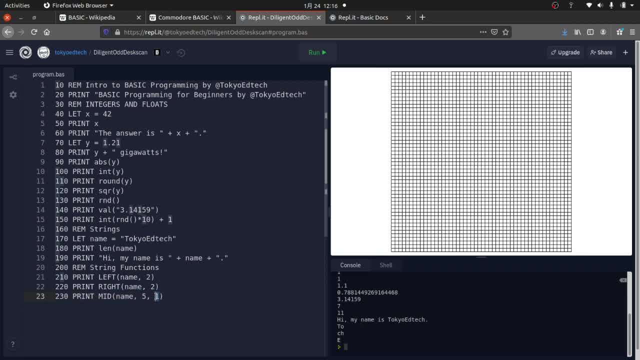 So that would give us e, because e is the fifth character and we only want one character at a time, I'm going to put that back to two, So that would be like a slice in Python. Okay, Yeah, that's pretty cool. 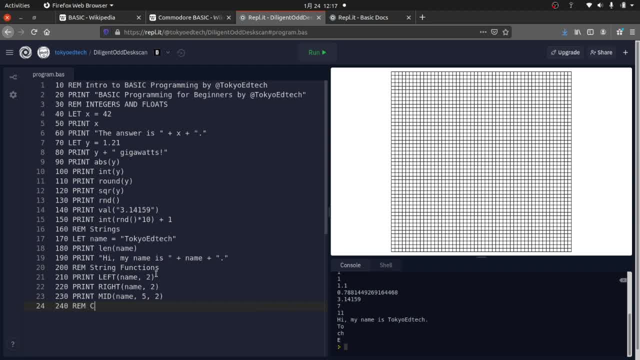 Next up is we want to go ahead and do conditional statements, And these are if statements. So, for example, watch what I do here. I'm going to say if- and this is very similar to what we've been doing. let's say, if x equals 42.. 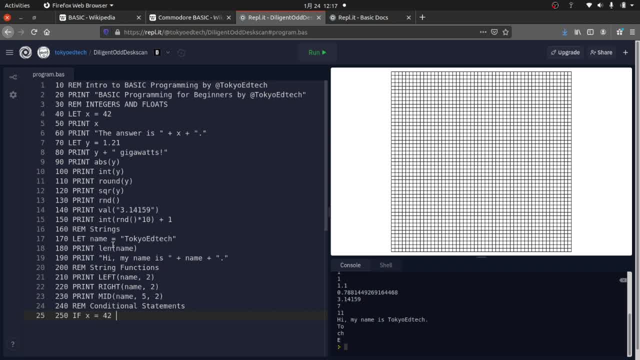 Now notice: it is a single equal sign. Okay So in pi, or in basic, Okay. So when you assign a value, it's one equal sign. When you compare values, it's one equal sign. In Python, it's one for assignment and two for comparison. 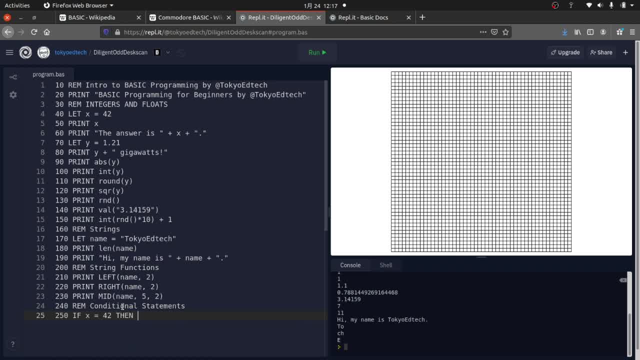 So here is the format. If something, then something else. So I'll say print 42. And I can say else: print 42. Okay, So you can see how we've got. if then else, and it's all one line which is kind of interesting. 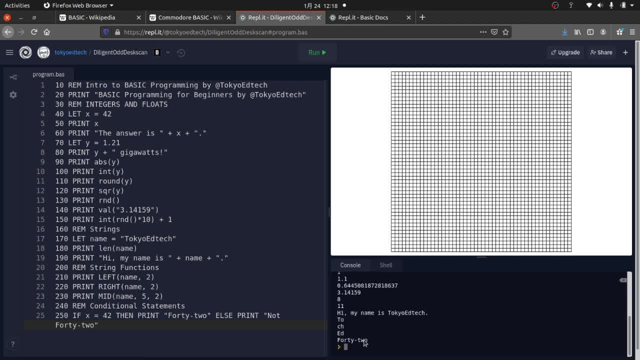 Okay, So I'm going to go ahead and run that. And so x was 42. Let's go ahead and just change it, just to see what happens and make sure it's working as expected. Okay, Not 42.. Now, in basic, I'm going to put that back to 42 because that's a more important answer. 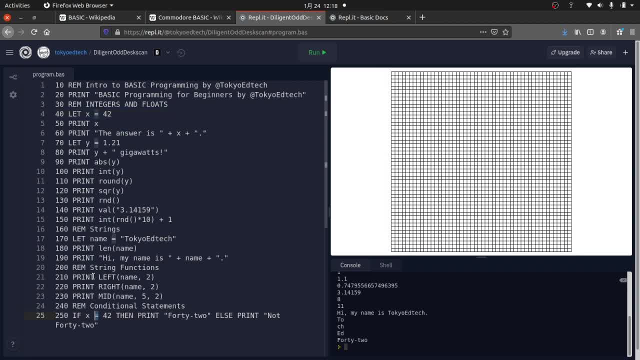 In basic not equals, It's like this. That is the old school kind of basic way of saying not equals. In Python it would be exclamation point: equals, But in basic it's like this: You can also do greater than you can do less than you can do greater than or equal to. 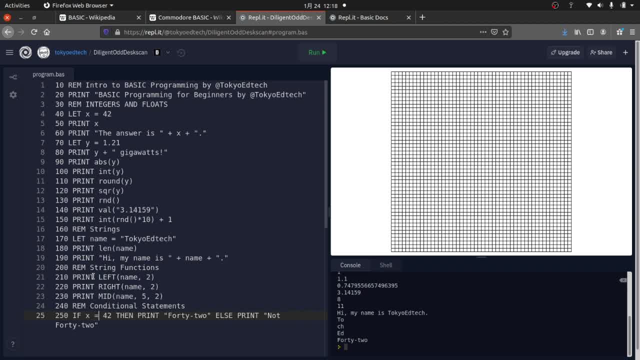 or less than or equal to. So it's very similar to modern programming languages, except for the not equal to is a little bit different than probably what you're expected to. Okay, Moving on, Okay, So we're going to do so. 60, we're going to or 260, we're going to do loops. 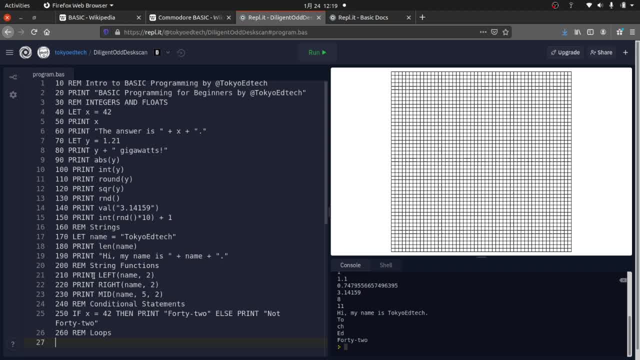 Okay, And again, depending on the basic variant you may or may not have while loops, I think a lot of the early basics just had for loops, but so I'm going to go with that. So I'm going to say 270, I'm going to say 4i equals 1,, 2,, 10.. 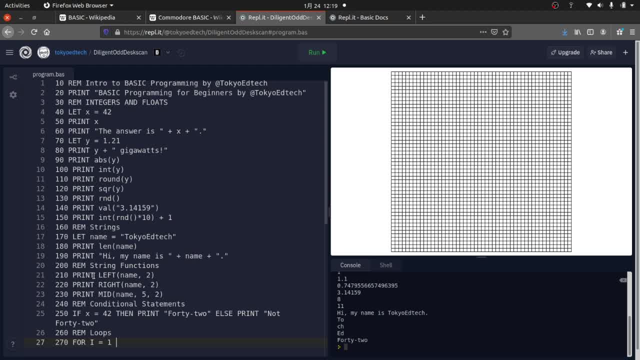 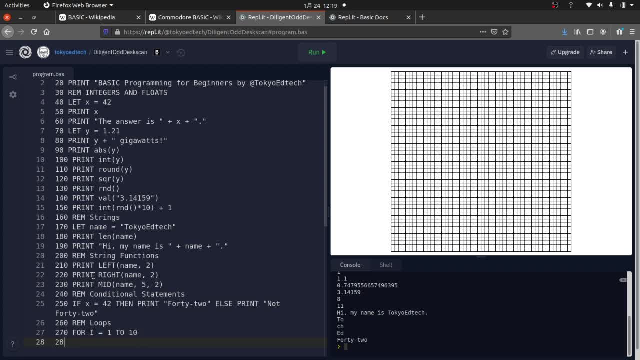 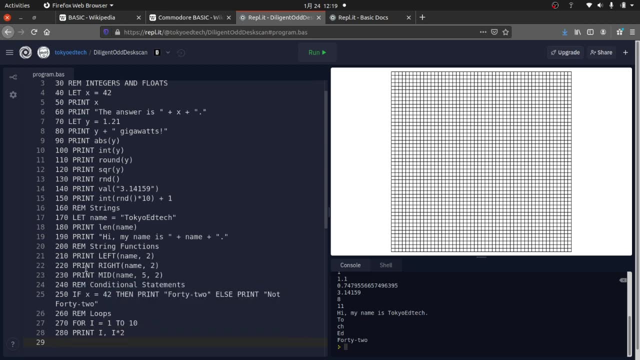 I'm going to go ahead and hit enter 280, I'm going to say print i. I'm going to try i times 2 and just see what happens. I haven't tested that one yet. And then 290 is going to be next i. 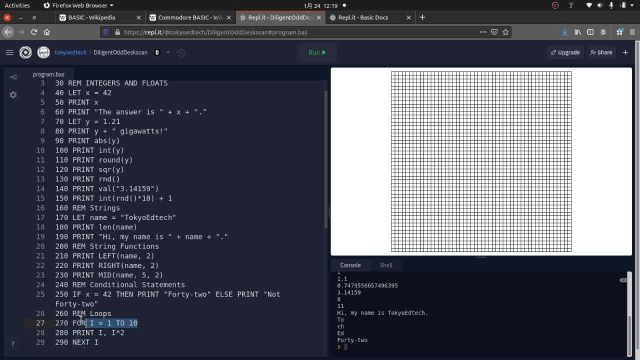 Okay, So a loop, so a for loop at least. so a definite for loop starts here. So we have a variable, we have a starting value and an ending value. We can also add step if we wanted to like, step two, for example. but let's try that. 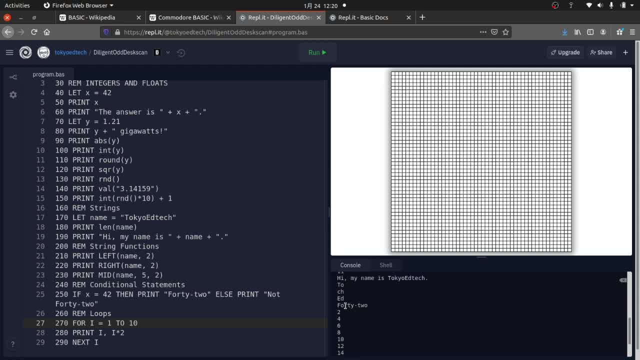 and see what happens. Okay, You can see 2, so print i comma: i times 2.. Okay, That part didn't work. So what I think I have to do is print i plus, quote, quote, plus, and I'm going to put times. 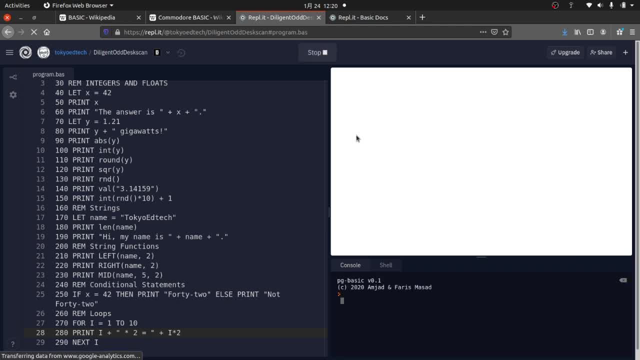 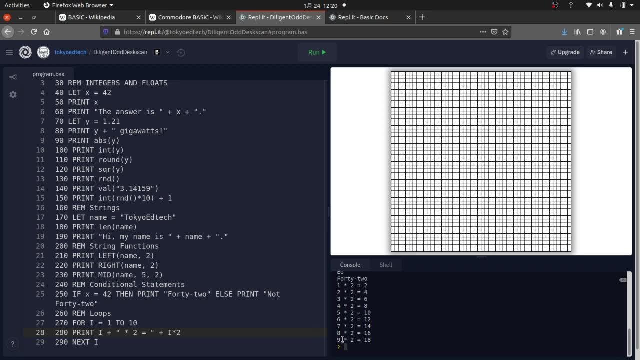 2 equals, just for fun, and go ahead and see what happens. Okay, 1 times 2 is 2,, 2 times 2 is 4, et cetera, et cetera. Notice it stops at 9.. 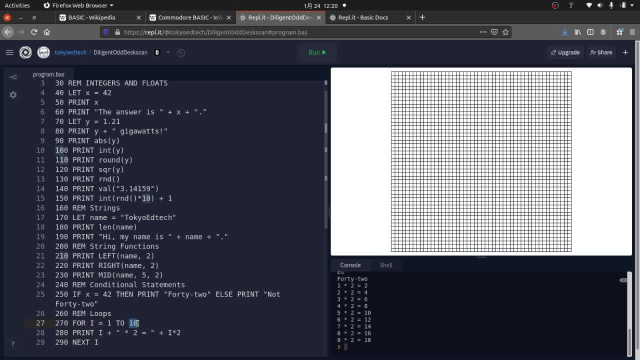 Okay, So that's just the way Python works. If Python works as well, it will stop at 1 minus the maximum value here. Okay, And then you can see here I just used a print statement to kind of print that out nicely. 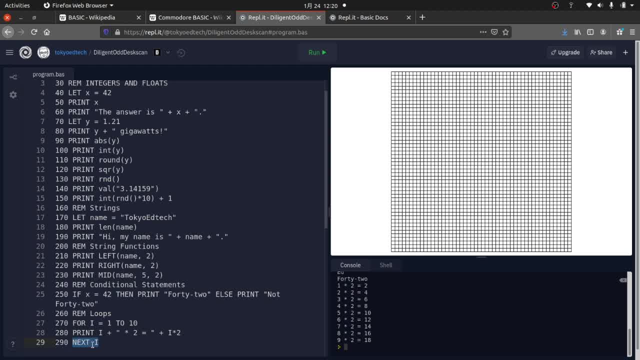 And then you need the next i to tell it where the end of the for loop is Now. in Python you would indent, or in Java you'd have a curly brace, but in basic you do not. So you can see how basically all these same concepts exist. 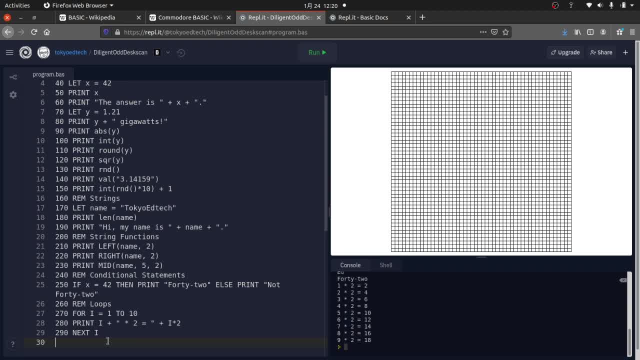 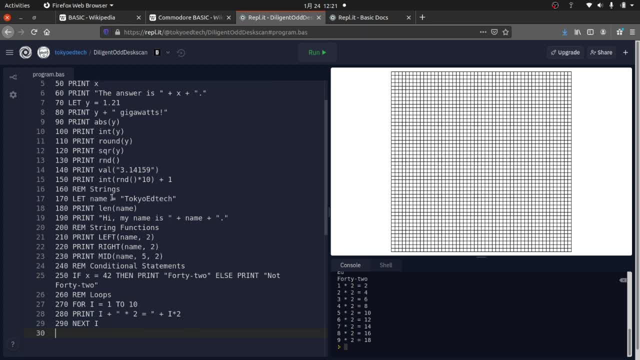 Well, not all of them, But the basic concepts exist, but they're just done a little differently. And again, these line numbers are a little bit weird. We haven't really used them yet, but we're going to in a little bit. 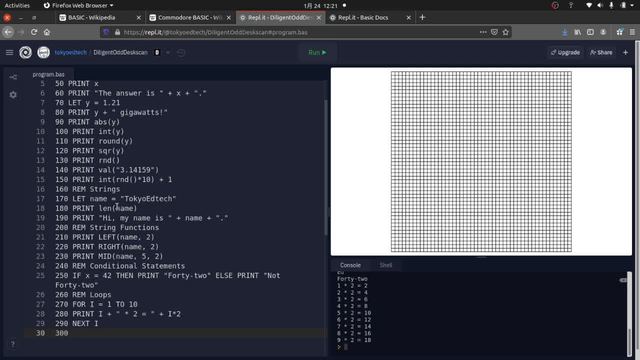 Basic also has arrays, So this would be like a list in Python or an array in Java. So go ahead and do arrays. Now, this is something that varies widely from programming language or from basic version to basic version. Okay, So in the old school kind of basic you had to do something called dimension. 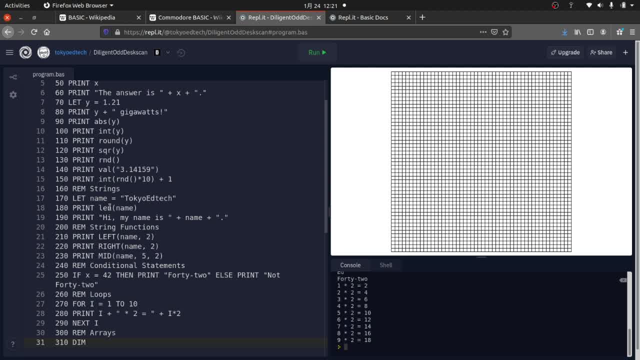 So you would have to do like dim, you know x, and then I forget the exact syntax and like say 10.. So you would say, okay, I'm going to have an array called x and it's going to have 10 spots. 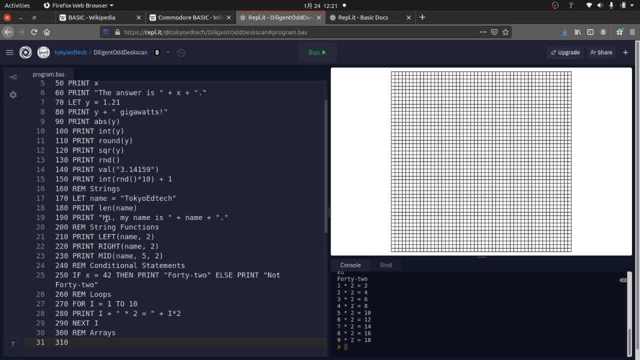 So zero through nine. This particular version of basic doesn't require that it has its own command called array. And I'm going to call this scores Also, just just you know, like a lot of the early versions of basic, you couldn't 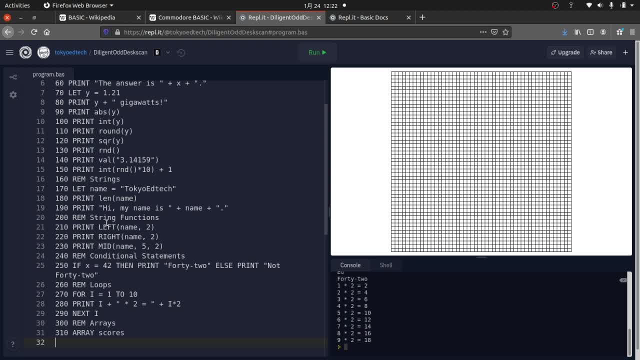 do like multiple, like the really really early versions. I don't think you could do multiple characters in a variable name. Everything was like a, b, c, d, e, f, g, I think. don't quote me on that. 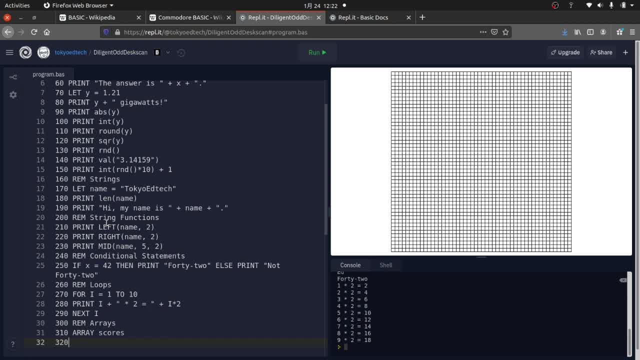 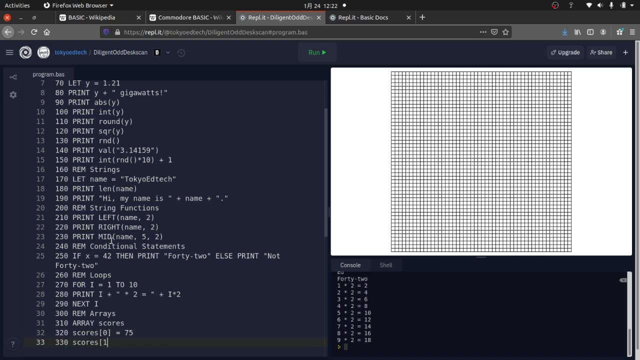 So yeah, so I made an array called scores, And then what I can just do is just probably what you're used to: Scores zero equals 75,. scores two- uh, oops, I missed the zero. Scores one equals 85, and scores two equals, let's say, 95.. 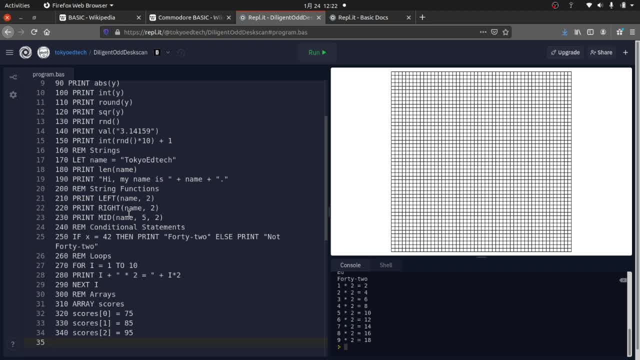 And then what I could do is- just like we're used to, probably in other languages- print- oops, that's a, that's a hard habit to break um scores, that's print scores. let's say, I want to print scores one and I should see 85.. 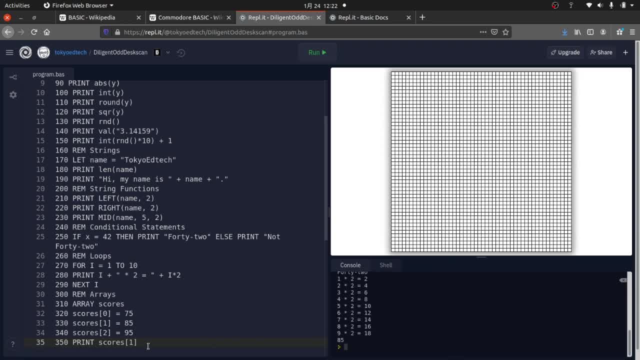 And we do see the 85, and this is where I could use a loop. I could say for i in range zero to three, and print out all the scores, just like I would with a list, say a list in Python. Okay, 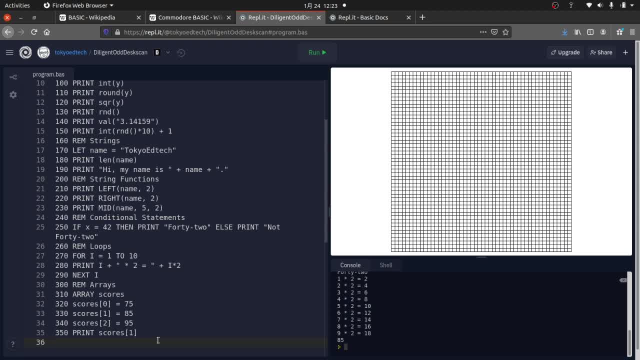 Um, so yeah, that's, that's kind of the basic, basic stuff. So probably if you're thinking to yourself, well, what about functions? And this is where this is a really big difference between, like old school basic and, say, modular. 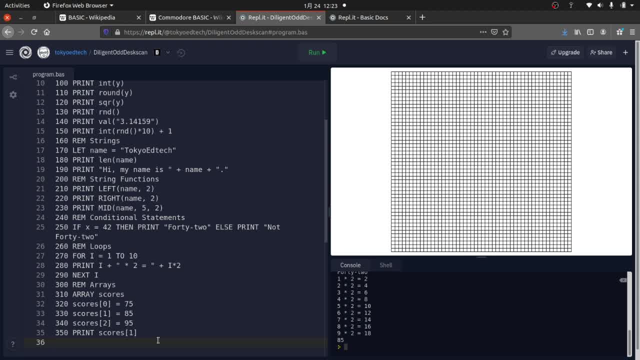 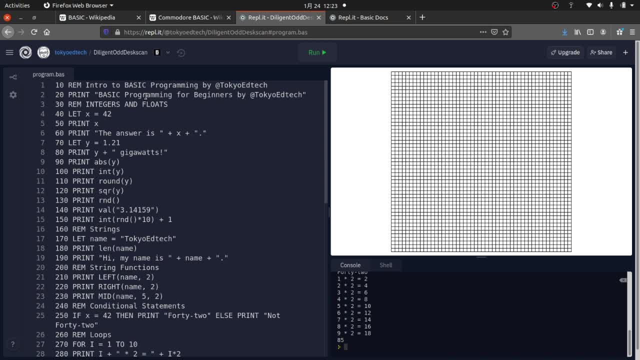 functions. So you're gonna be able to use old school basic in modern programming languages. Um, something you you may have noticed here is that all variables in old school basic. now there are new, there are modern versions that don't follow this, but this old school. 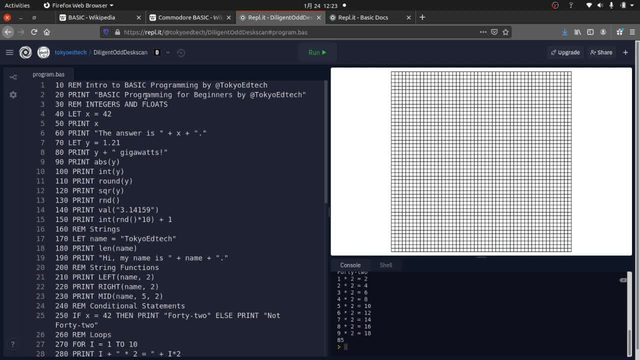 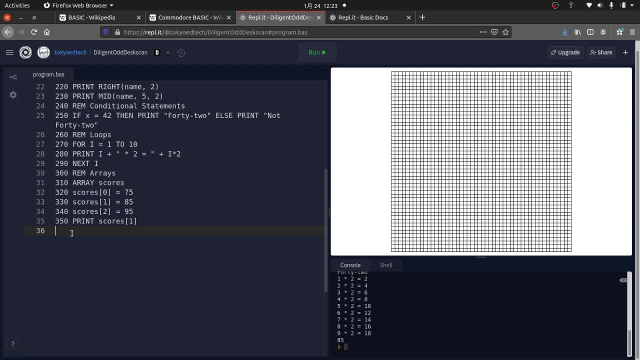 ancient type of basic. all variables were global. Okay, So, yeah, just just think about that, I'll just, I'll, just I'll leave with that thought. Um, so we couldn't really make functions do was make subroutines. okay, so, for example, I'm gonna make a subroutine and 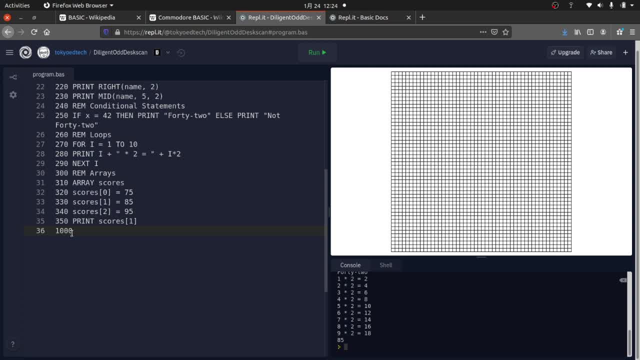 what kind of standard practice was was to put it way down farther in the line numbers. okay. so for example, I can say: print this: you know this is a subroutine. and then, after you did a subroutine, you put return. so how this worked was: I would do 360 and I say RAM subroutines and I'll say 370, go sub. 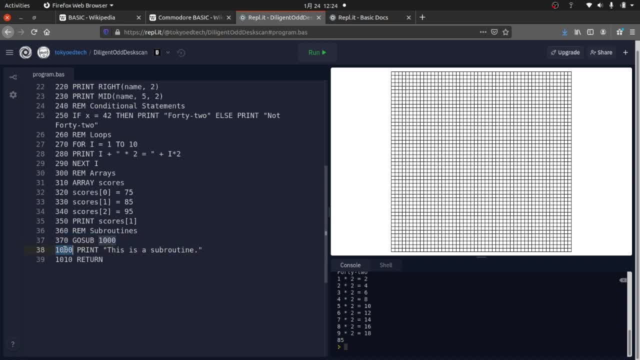 1000. so this line number here. so this means go to the, the subroutine located at 1000.. So think of this as a function. I jump down to here and then, when the function is done, I return. Now, note, I am not. 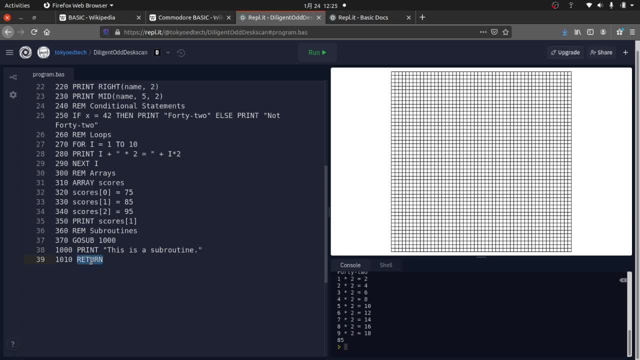 returning a value. This is a very different statement. All this does is, when the subroutine is finished. the subroutine can have 100 lines, doesn't matter. When it's done, jump back to where we started, And then what I'll do is here: 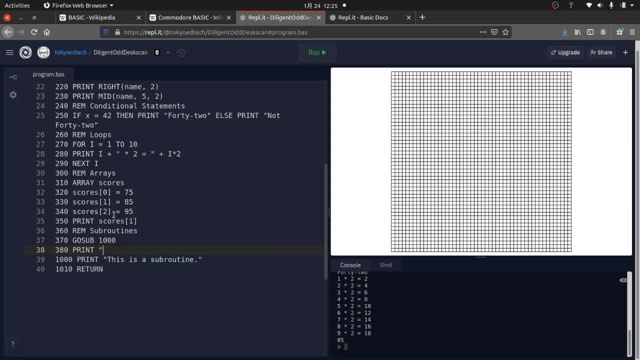 I'll say 380, print back to the main program And then what I'll do is I'll go ahead and put line 990 in there end, So it ends the program. So I'm going to go ahead and run that. I'm going to make that a little higher. Sorry, I should have done that earlier. 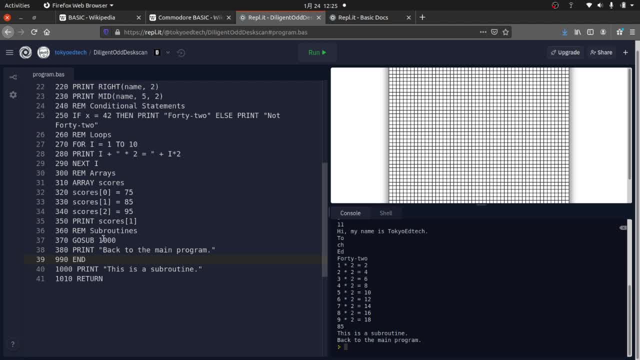 So you can see we printed our 85.. We got to go sub 1000. So the program jumps down to 1000, prints: This is a subroutine, So I'm going to go sub 1000. So the program jumps down to 1000, prints: This is a subroutine. 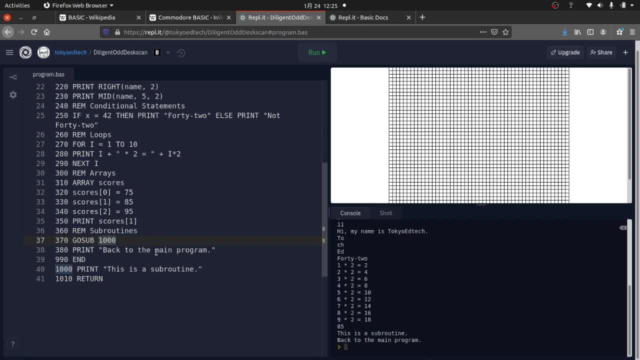 Returns back, goes to the next line, prints back to the main program, and then we end it. Now, if I didn't have this end in here, it would print this as a subroutine again. We'd probably get an error, because there's nowhere to return to. 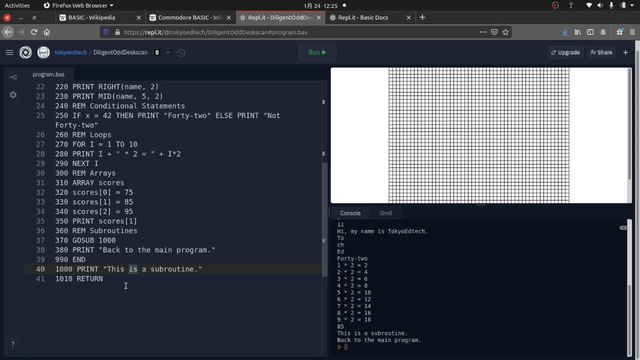 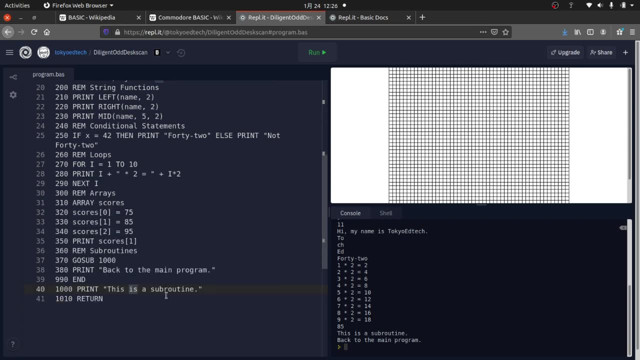 Okay, so that is how subroutines work, which is the modern or the old-school equivalent to functions. But if you notice, you can't pass a value to that because, as I mentioned, all variables are global. So yeah, it's just so this. 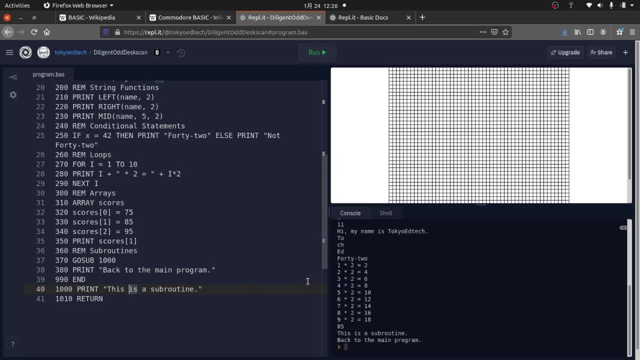 this led to what was called spaghetti code, And we'll talk a little bit more about one of the other jumping statements called go to in just a minute. The last thing is, or one of the last things is, user input. So how do I get input from? 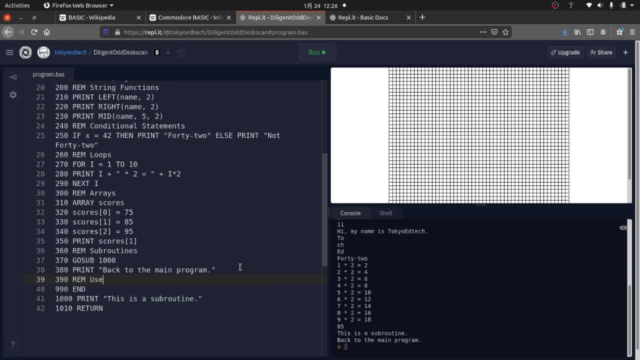 the user 390, REM, I'll say user inputs. So what I might do is ask the user for their name, Okay. so if I want to do something like 400, say name, sorry input, Okay, what is your name? I always like to put that little thing in. 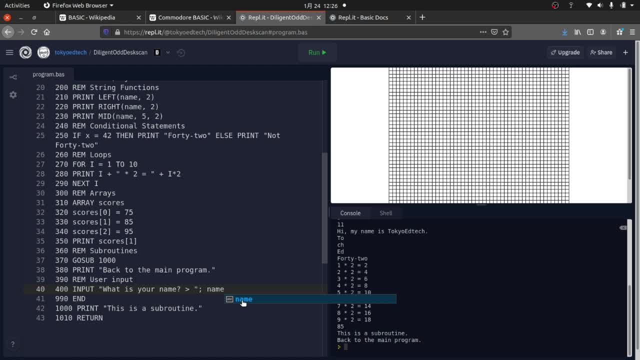 there And then watch, it's a semicolon, and then the variable name, Again on Commodores. this would have to be a dollar sign to tell it's a string. And then 500, oh sorry, 410,. I could just say print. you know, hi name. 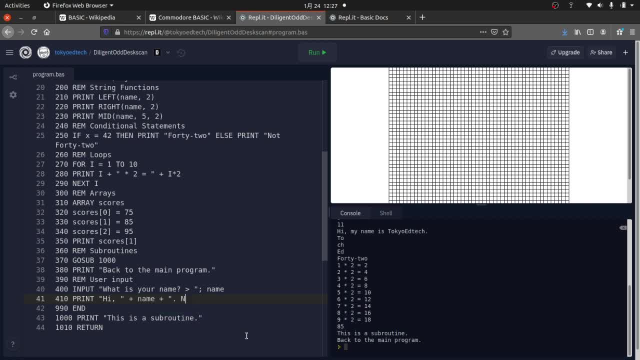 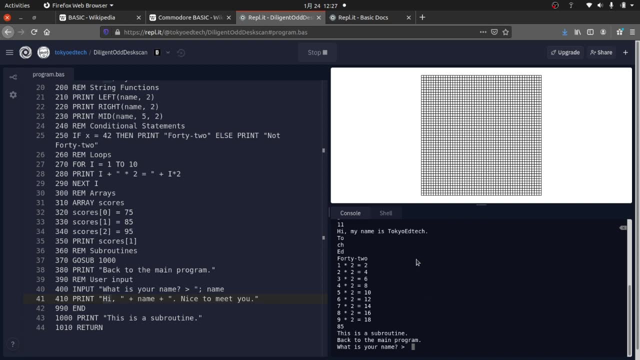 very nice to meet you. And then, yeah, let's go ahead and run it. So what will happen is the program stops, just like it does, like I said, in Python or some other programming languages. Usually we have an input and you input whatever it is. So my 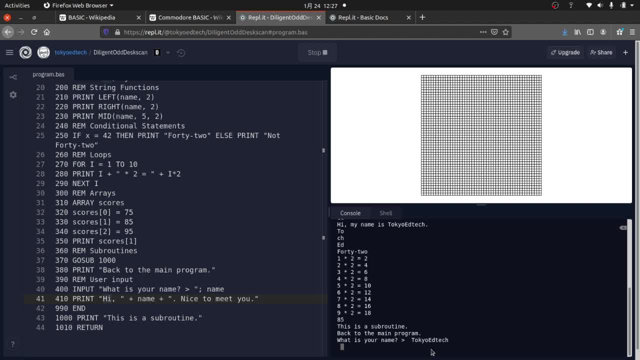 name is Tokyo, Tokyo, EdTech, and it's gonna say something: nice, Hello, Tokyo, EdTech, nice to meet you. And then what I can do here- and this is the last thing- is I can use the same concept. I can say something like 420, haha, 420, input. Would you like to continue? 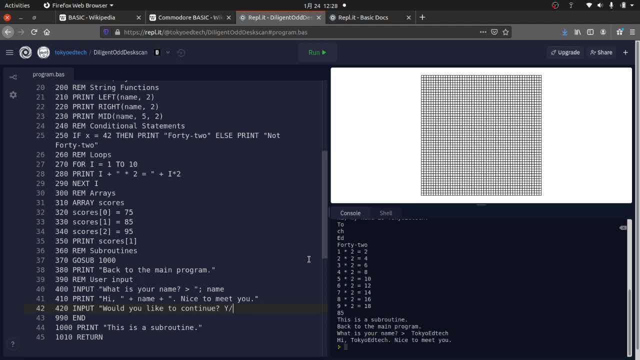 And usually you put like yes, no. And then I might say: you know, continue, That might be a keyword, So like say c-o-n-t for continue, And then I might say 430, if cont like continue equals y, then go to. 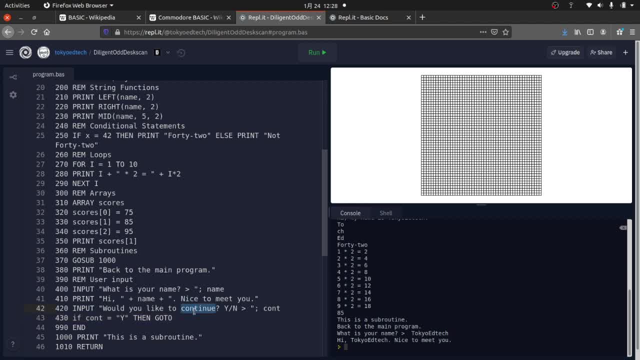 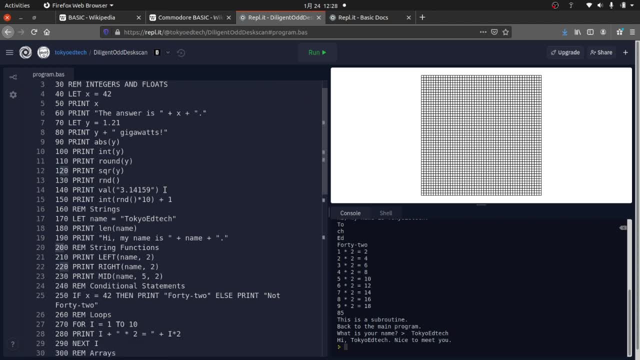 I say, instead of continue, maybe try again, but go to, and then basically what I'll do is I'll go back to the start. And so what I want to do is I need a line number, So I would say go back to 20.. 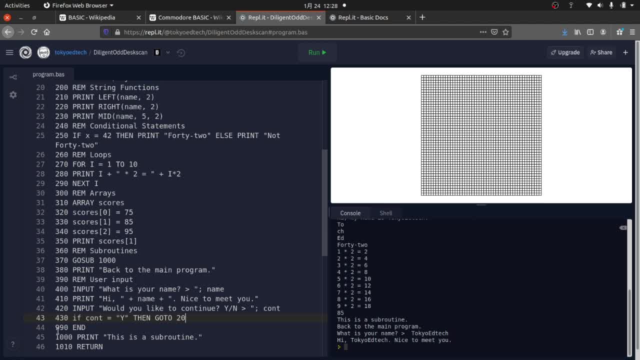 Okay, Okay, Okay, Okay, Okay, Okay. If it's not, then we'll just go ahead and end. So it's gonna ask me for my name. I'm gonna say Tokyo EdTech And hi, nice to meet you. Would you like to continue? 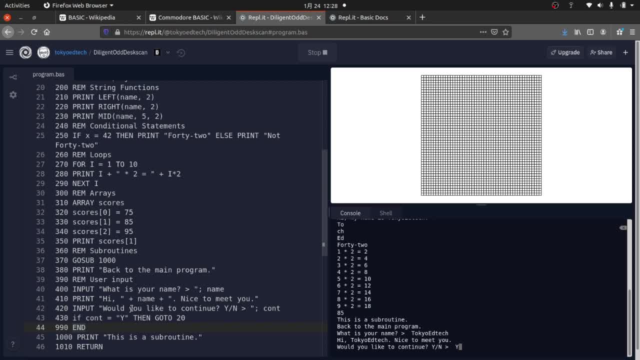 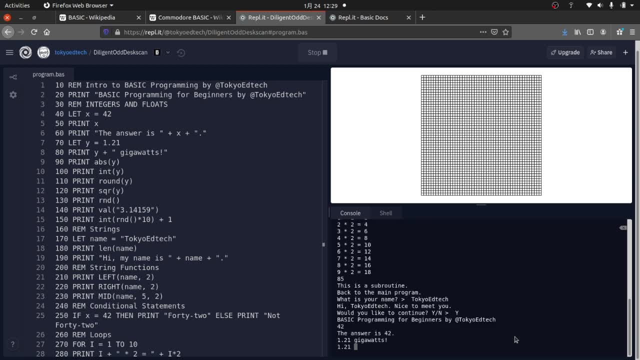 I'm gonna type yes, And what it should do is jump all the way back up to here. So this is how you would do, like a wild true loop. essentially, You just do a go-to statement. Okay, you see, it did it again. And Tokyo, EdTech And this: 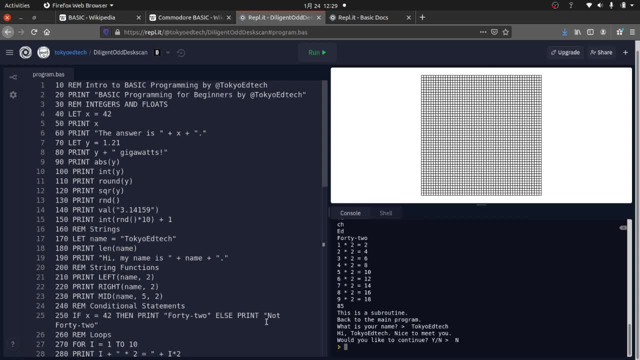 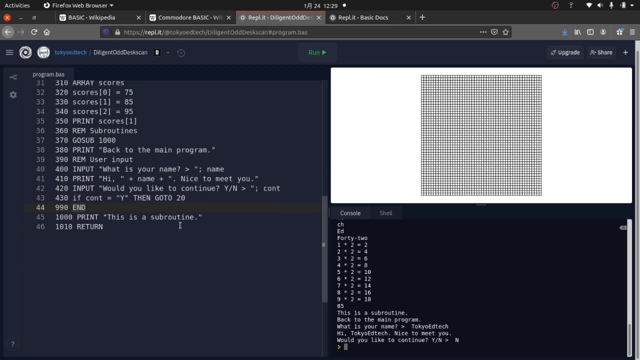 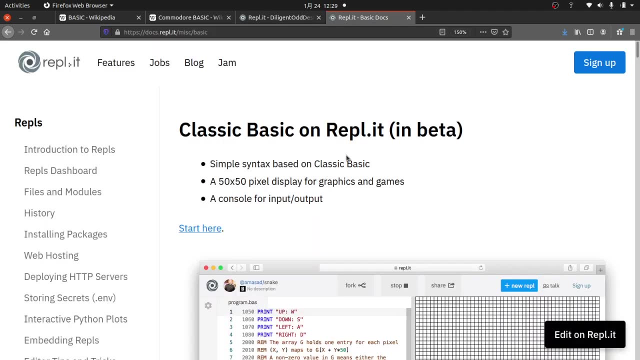 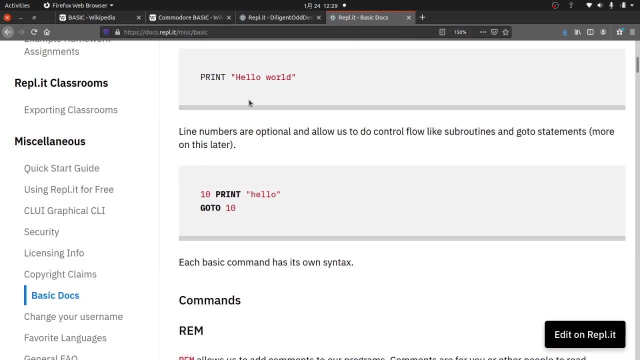 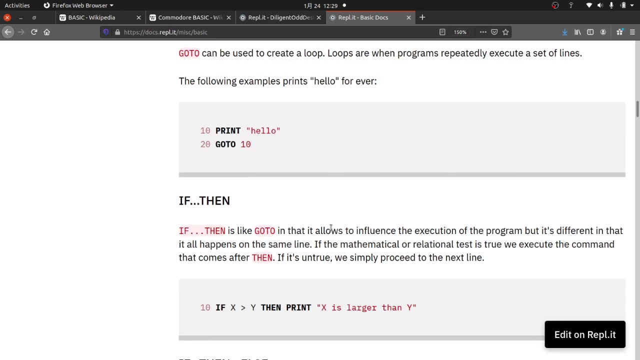 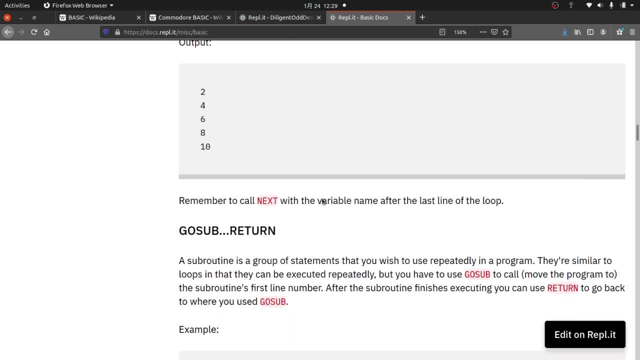 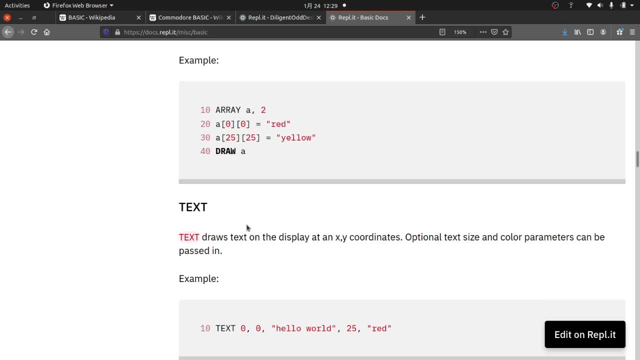 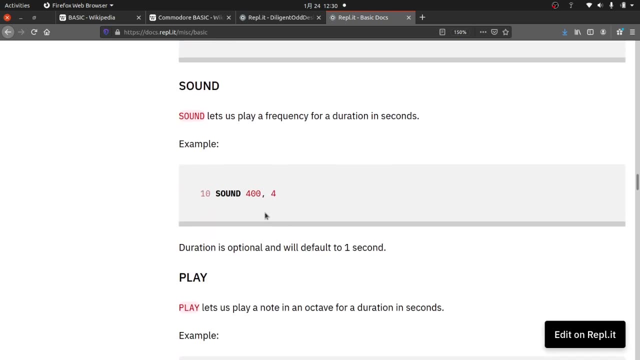 step. and next we talked about step. we didn't really do it- go sub and return, which we just talked about. this also has plot, display, draw, there's there's a bunch of different commands that are specific to this version of basic, so you can actually play some sounds and things like that. so it's pretty cool. and then 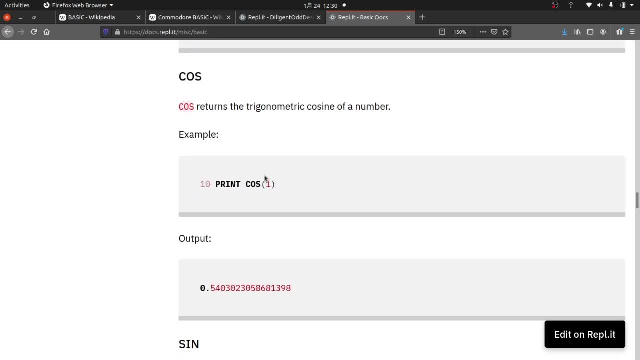 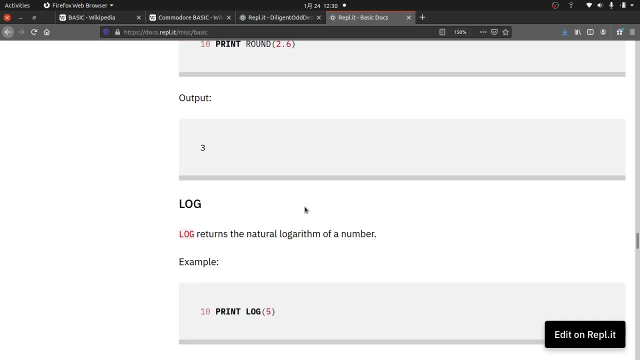 there's some built-in functions. we talked about ABS, ABS. I didn't talk about cosine sine, but it's there as well, so you can kind of look at this page and see some different things that that work. yeah, it's pretty cool. I guess whoever made this was really, really amazing and yeah, thank you for for making this and 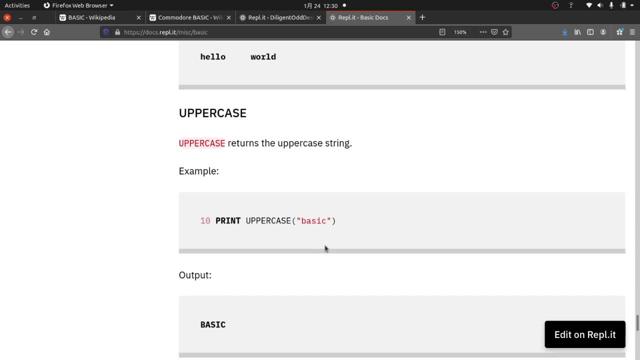 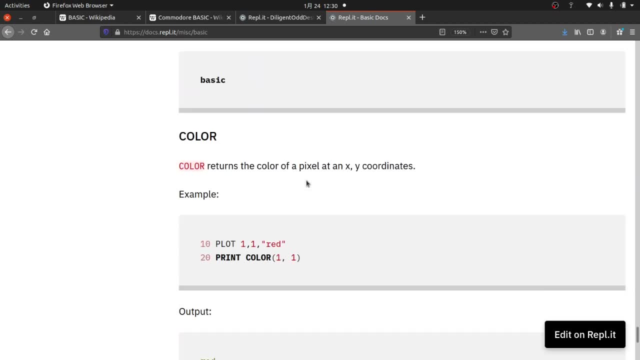 there's a few things probably that you know I left out, but I think that covers it. yeah, there's an uppercase which I don't recall Commodore basic having that. I think that was a little bit of a mistake but I think that's pretty cool thing. I know that wasn't common to all of them but it's probably. it's a very 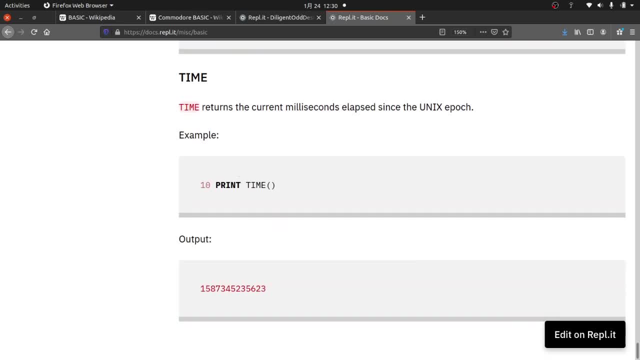 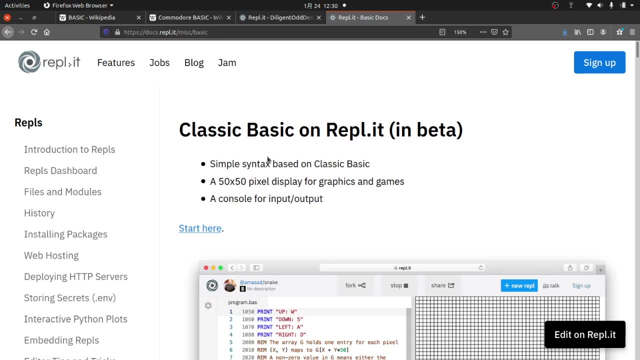 useful function and then you do some things with colors and getting characters and etc. etc. so, yeah, check that out for more details, but that's basically a nice overview of classic basic in yeah and on repli. it's really nice to them to have this again. you have to make a. you have to make a, I'm gonna 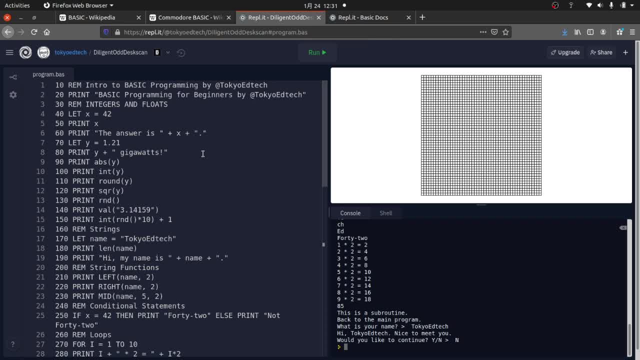 put it, you have to make an account, but you can go around, go around and look at can go right, go ahead and play with this. now what I do is I'm gonna go ahead and copy this and I'm gonna save this somewhere. I'll put this into, I'll put a. 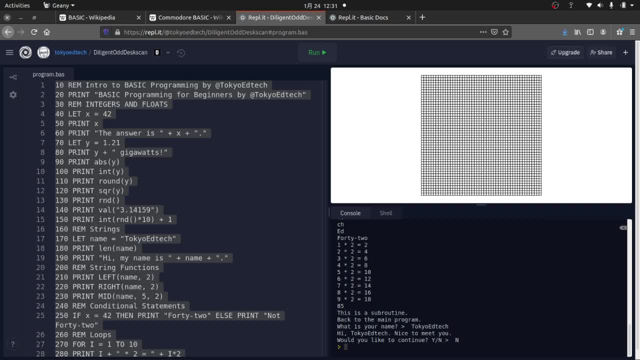 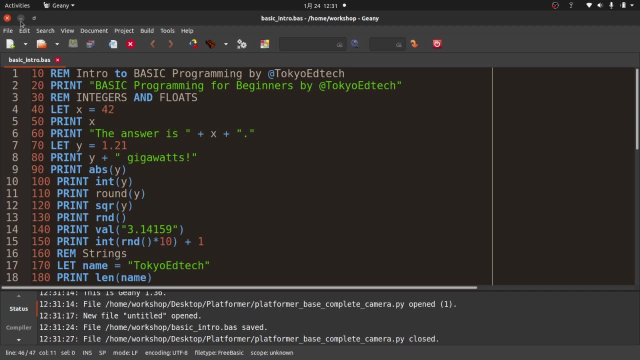 link to this down below somewhere and I'm gonna save that as basic intro basic. that's really unfortunate that the color coding doesn't work, but this is what the color coding looks like in genie- unfortunately, in genie, I can't run this because I don't have a basic interpreter on my computer. so what I want to do 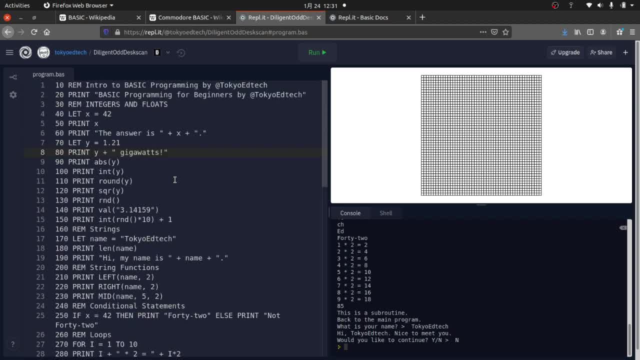 I'll tell you. I'll just make a quick separate video for that. I was gonna do rock-paper-scissors, but let's stop this one and I'll make a quick separate video for that, okay. so, yeah, thanks for watching. I hope you enjoyed this little trip down memory lane and you can see how coding used to be done. this was.